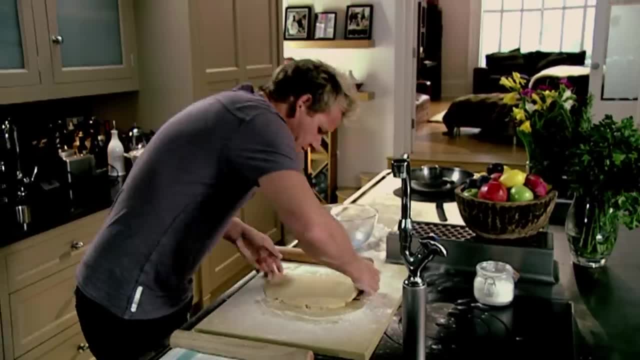 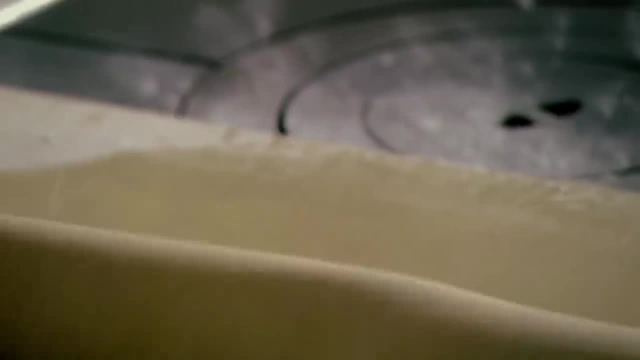 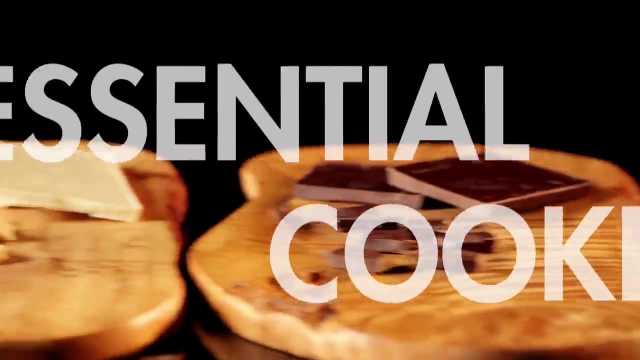 it sort of unites the pastry. immediately Apply pressure, Turn the pastry. Now the average thickness is down to a one-pound coin. Back on to the rolling pin And look Beautiful For the neatest edge on tarts and quiches. 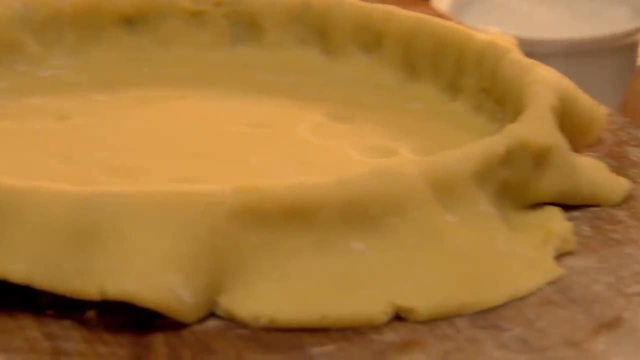 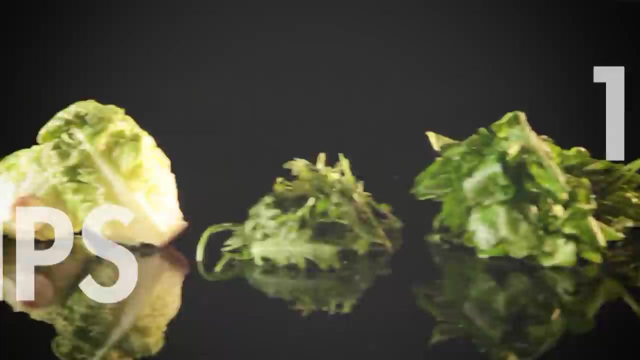 my tip is to let the pastry hang over the side of the tin when you bake it. Trim around the edge. once the pastry is cooked, It will give you a cleaner edge and prevent it from shrinking. My tip for even rising is to place cakes and tarts in the center of the oven. 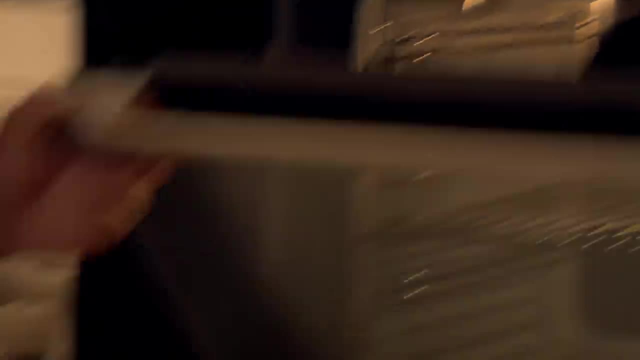 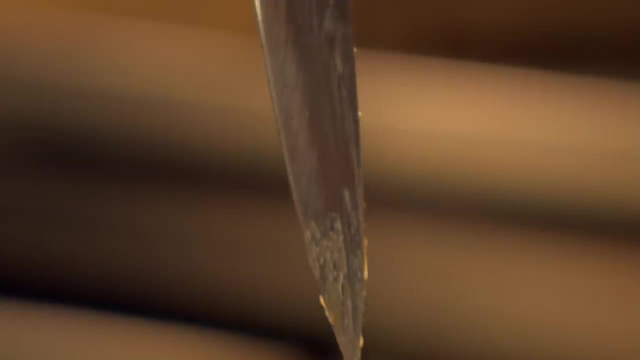 So the air can circulate all the way around them. To test your cake, to make sure it's done, insert a knife, skewer or even a piece of spaghetti in the center. If there's mixture stuck to it, it's not done yet. 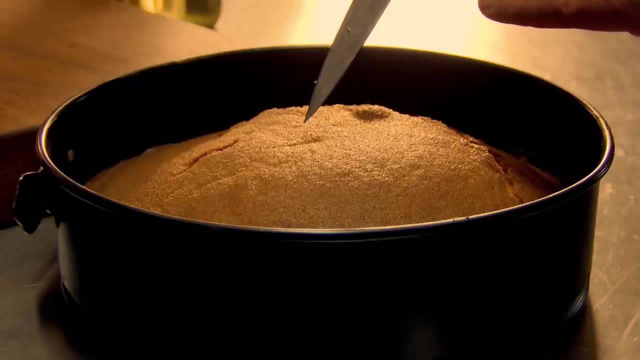 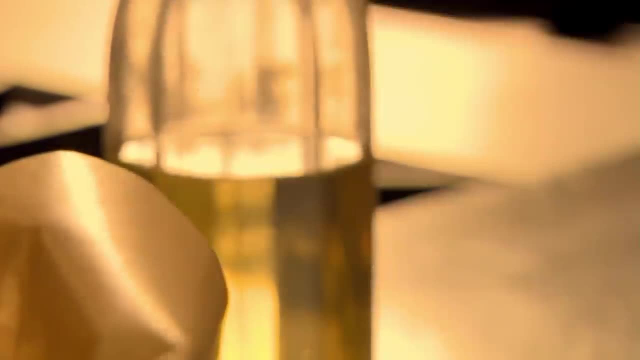 If it comes out clean, your cake's ready. If you don't have any baking beans to hand for blind baking, you can use any rice grain or pulse. You won't be able to cook with them afterwards, but do keep them to reuse them next time. 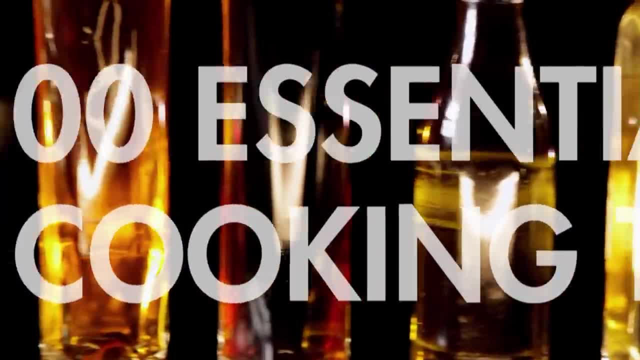 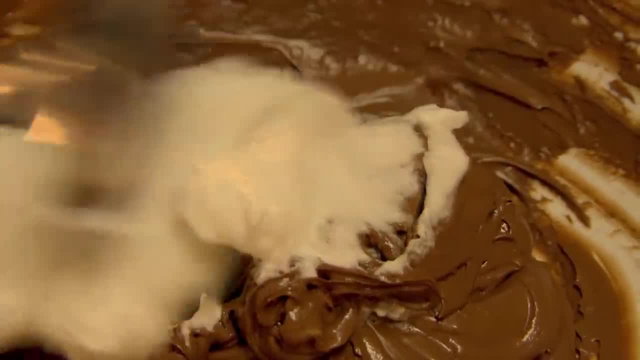 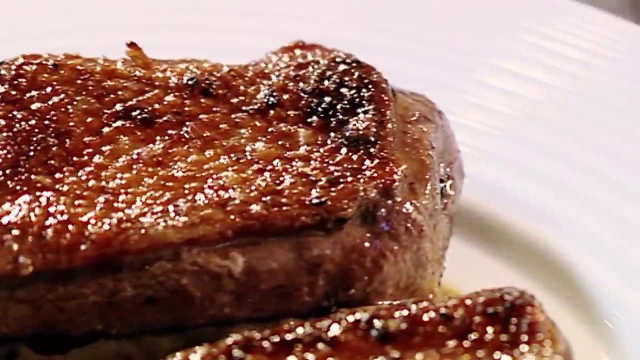 When you're folding egg whites or whipped cream into cake mixtures, you want to retain as much air in the mixture as you can. My tip: use a metal spoon, as the sharp, thin edge will keep more of the air. in Starting with how to cook duck breast perfectly, the slow way, 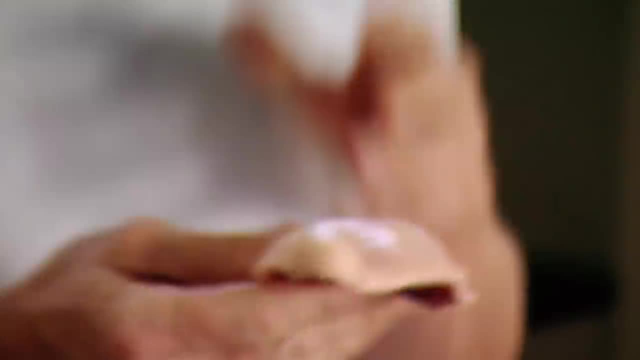 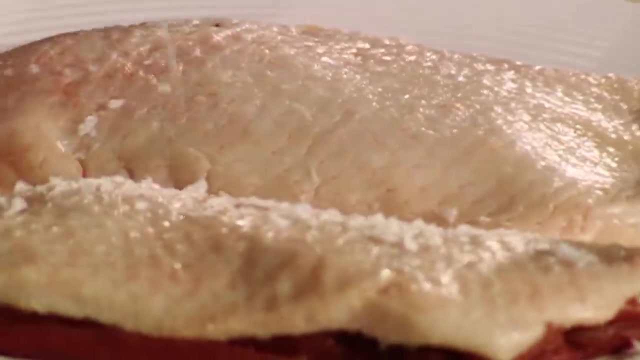 Duck breast. Never be scared about cooking this bird. Absolutely delicious, very healthy. First oven on 200 degrees And then salt pepper. Now the salt will help to extract the water out of the fat. Non-stick pan. 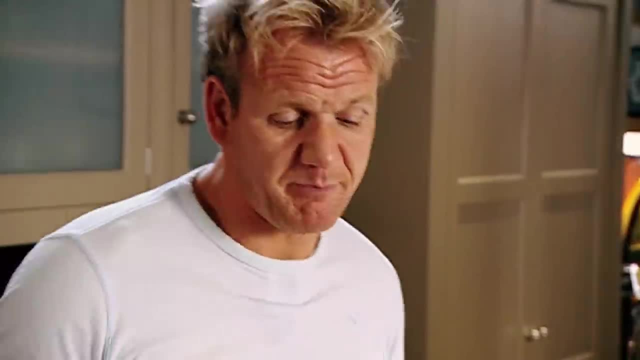 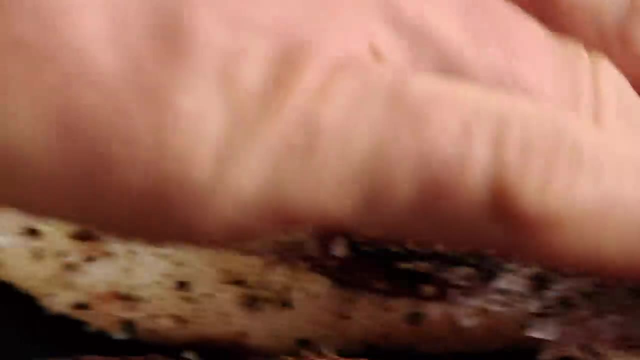 No oil But start the duck breast in the pan. cold Skin side down. It feels and sounds a little bit weird. But if you put them into a cold pan and turn the heat up gradually it starts to release the fat. If you put them into a hot pan, 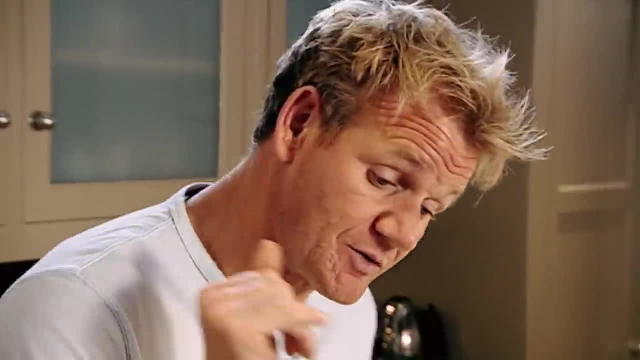 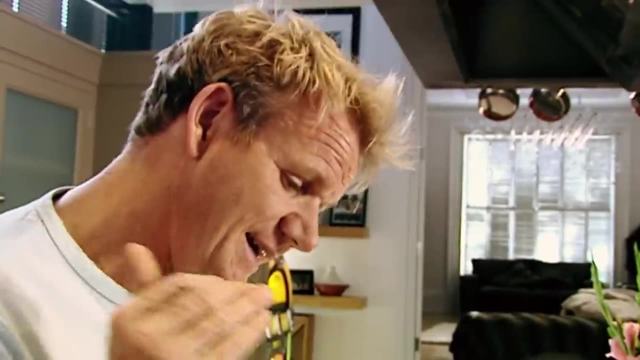 it seals them in and the fat stays in there. We want to render that fat down. 90% of that duck breast will be cooked on low heat. We want to make sure that the fat comes from its skin Keeps the duck nice and moist. 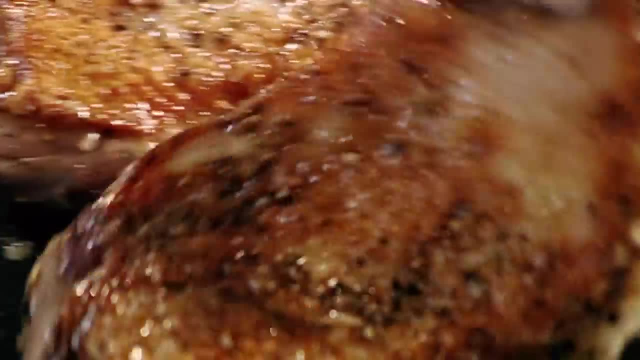 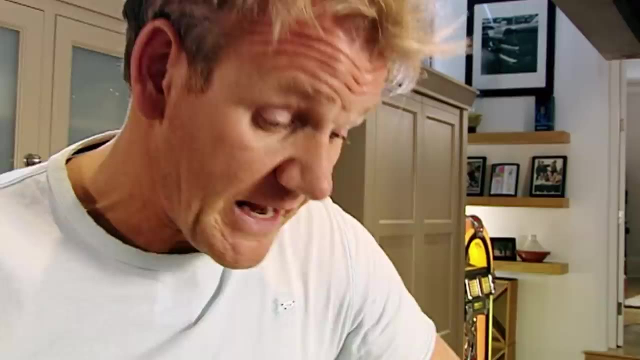 But more importantly, it stays crispy Once the fat comes out. turn the duck over Nice high hot heat. Seal the duck. Now they're going in the oven, Skin side down, 200, 6 to 8 minutes. 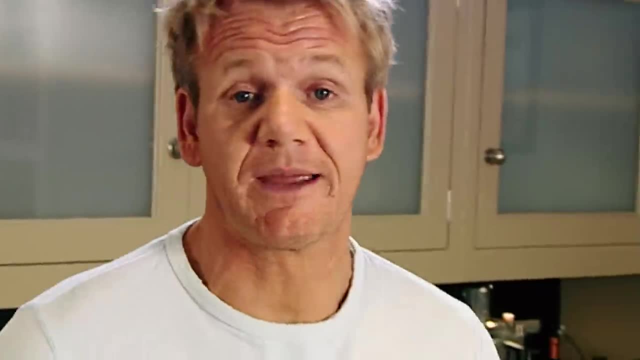 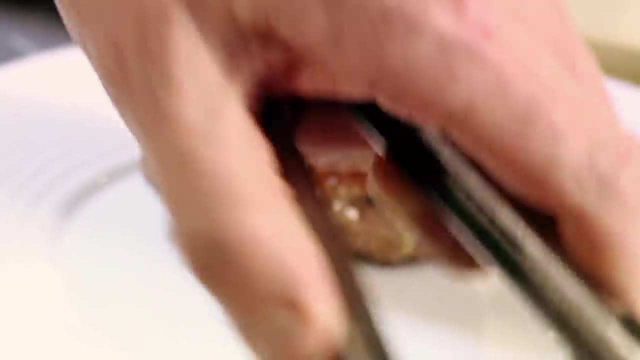 If your pan's got a plastic handle on it, then transfer the duck breast onto a tray, But make sure you put the tray into the oven to get hot first. Cooking duck is like cooking a piece of beef- You can't slice it piping hot. 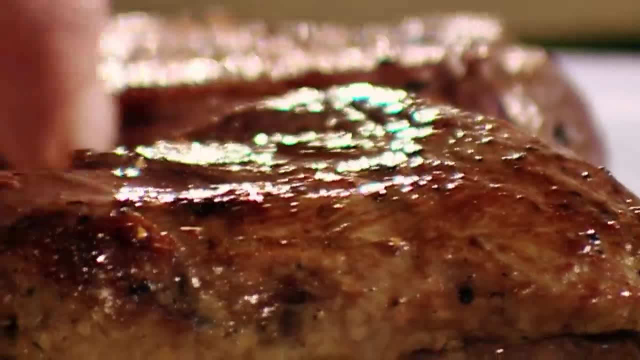 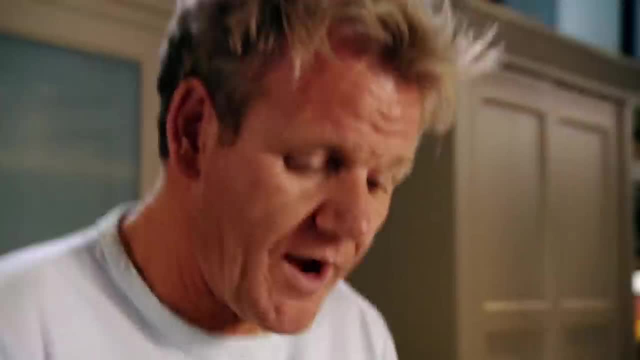 All the goodness runs out. Just quickly turn it over, Push your fingers in there And it's slightly resistant but still quite bouncy, And that confirms they're quite pink in the centre. But the important part now is leaving that to rest. 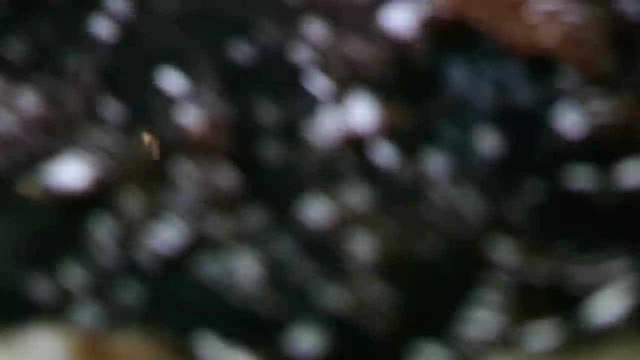 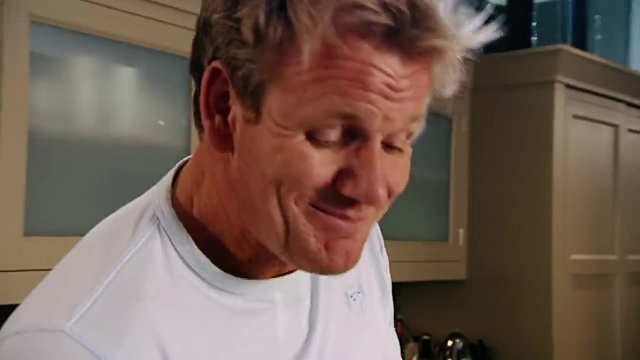 Let them cool down And then we'll slice them. Keep that excess duck fat, And there you go. Next time you're sauteing potatoes, you just take them to a completely different level. Now slicing the duck, just slice it at an angle. 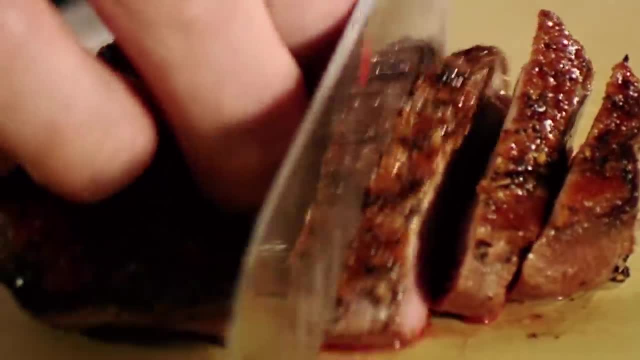 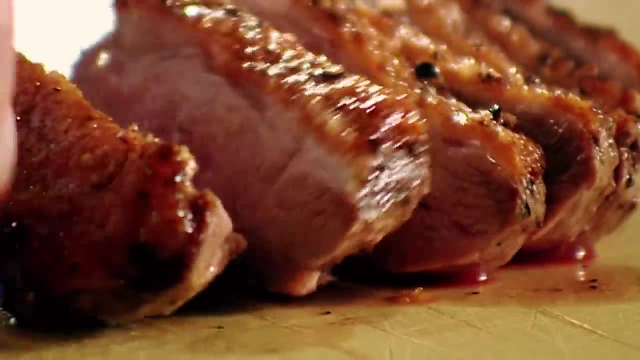 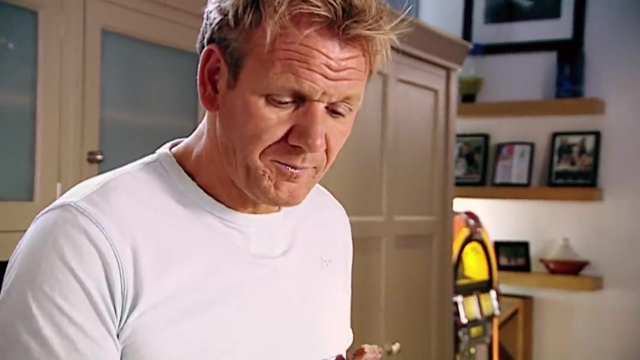 Not too thin. If you slice it thinly it goes cold quickly. So nice thick slices, Nice crispy skin on top And a beautiful clump Roasted duck. All the white fat gone, Nice crispy skin And absolutely delicious Mmm. 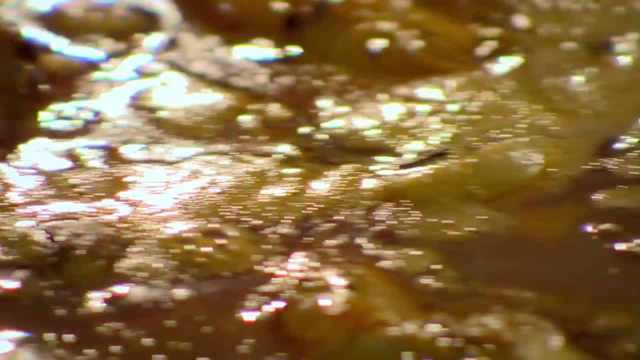 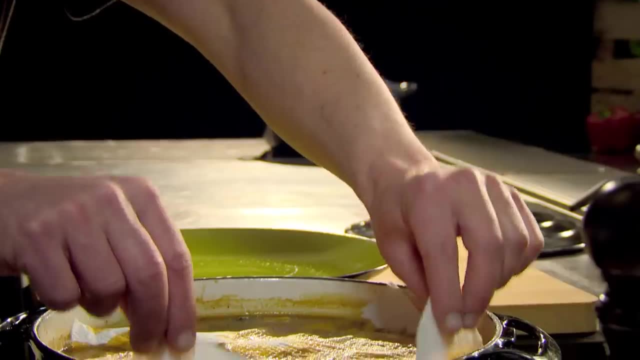 Another slow cooking tip is When slow cooking stews and casseroles, fat will rise to the surface. To get rid of any excess oils, my tip is to remove them with kitchen paper before serving. This also works brilliantly on gravies and sauces. 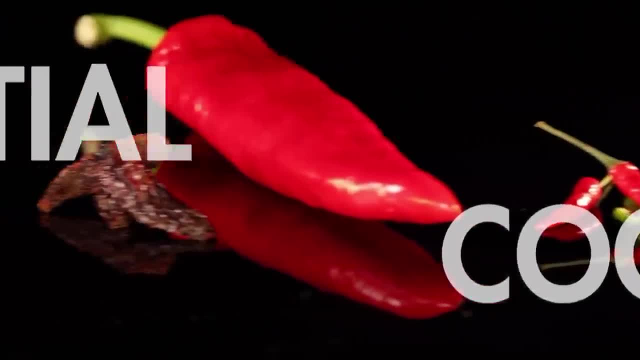 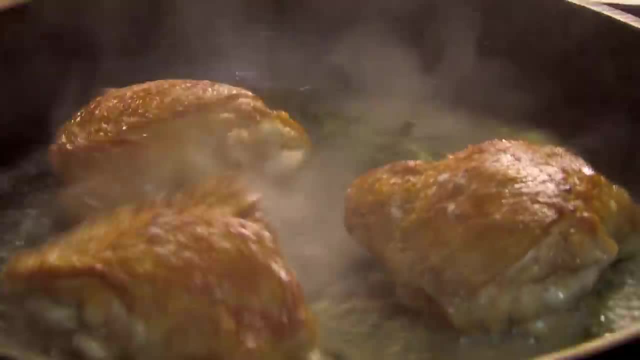 Many great slow-cooked dishes start by browning the meat. As the meat cooks, lots of flavours get stuck to the pan. To get it into your sauce deglaze with wine stock or vinegar. Never add soft herbs at the beginning of slow cooking. 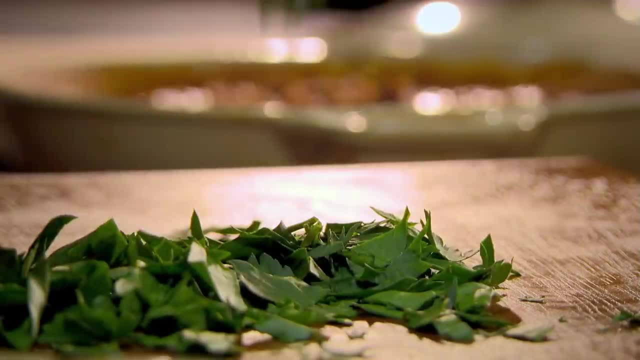 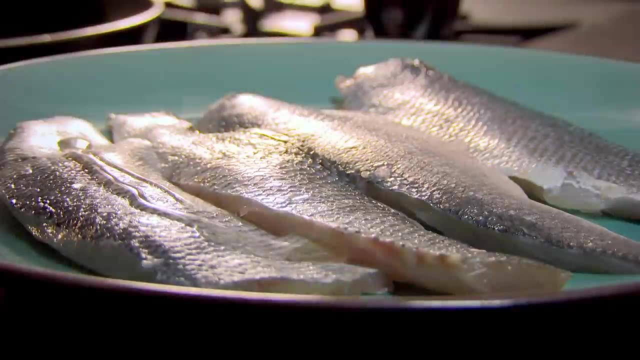 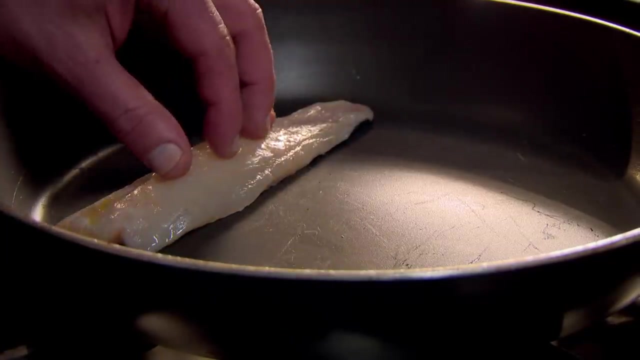 They're all too delicate. The tip is to add them at the end for that hit of fresh flavour and vibrant colour. A great tip when frying fish is to always fry it skin side down to keep it crispy And always lay the fish away from you. 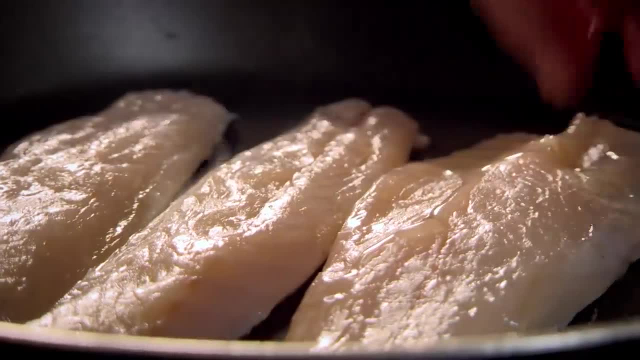 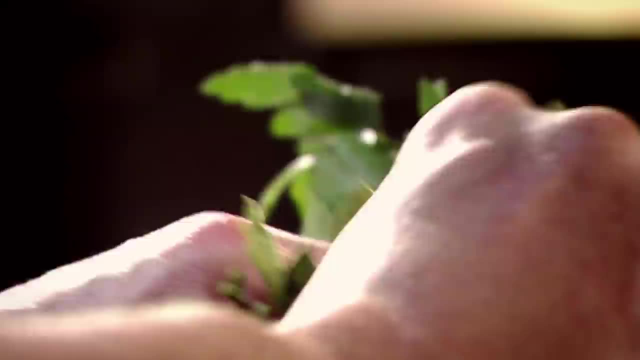 when adding to the pan to prevent hot oil from splashing towards you. First, how to make a fantastic chicken stock: a classic slow-cooked recipe that gets amazing flavour from simple ingredients. Chicken stock, The vital ingredient to good cooking. It transforms sauces. 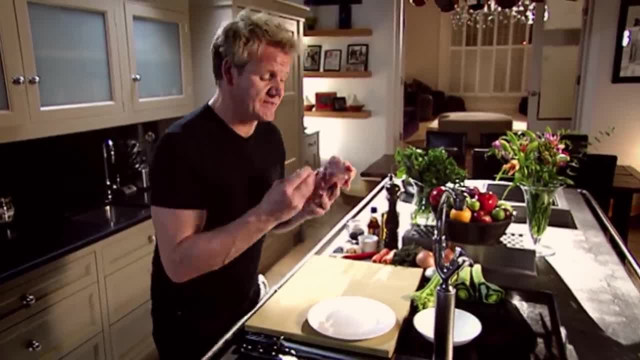 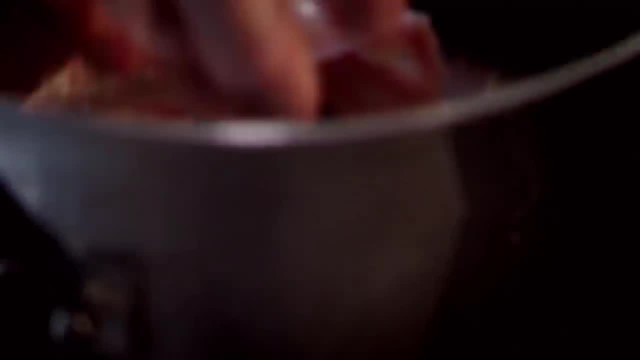 It's a fantastic base for soups And, more importantly, it's so easy to do A little bit of love and care at the beginning and it cooks itself Right. Step one: Chicken carcass into a high-sided pan, An onion. 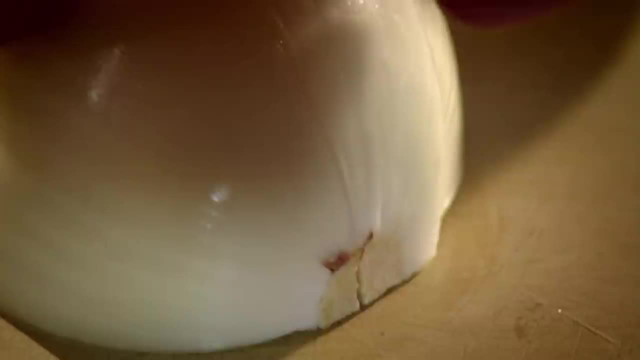 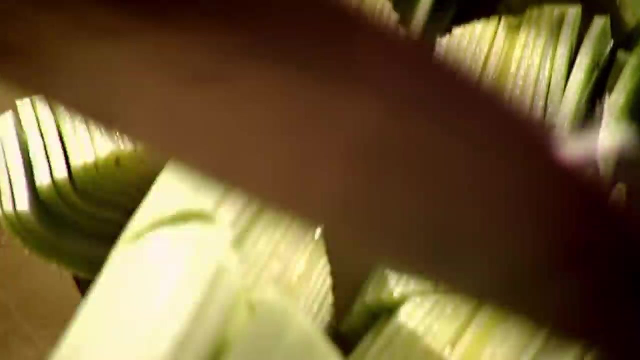 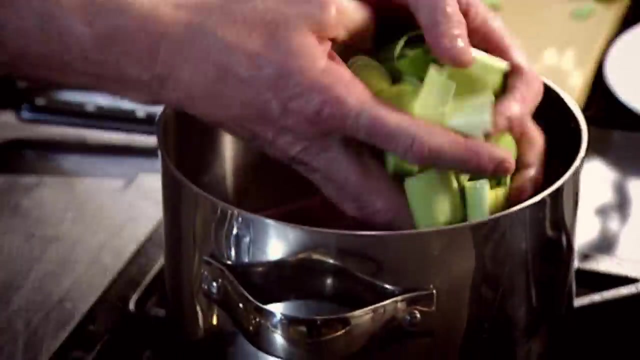 Doesn't need to be finely chopped. The vegetables flavour the stock Onion in, Then from there cut your leek into nice big, solid chunks, Roughly the same size as the onion. So all the vegetables cook at the same time. And then our carrot. 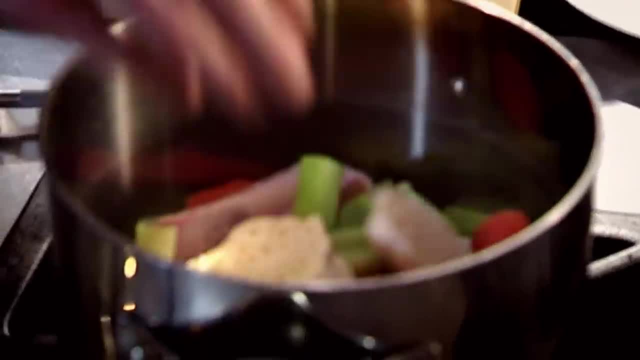 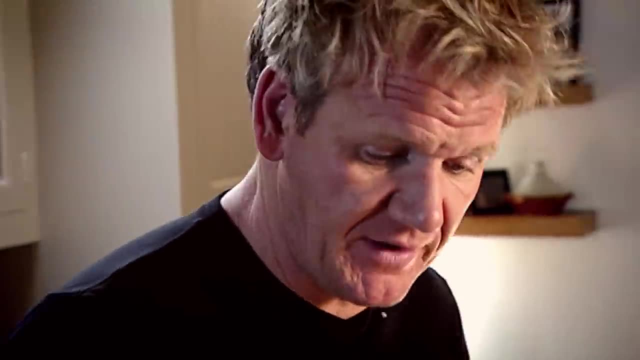 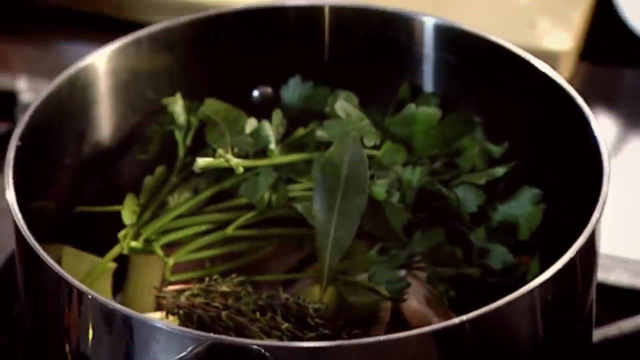 Celery in Garlic And then a nice sprig of thyme. That helps to really give depth of flavour to the chicken stock. A couple of bay leaves And some fresh parsley, And then peppercorns Pan and just lightly crush them. 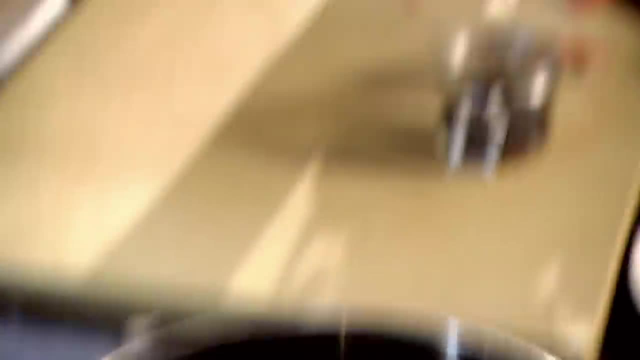 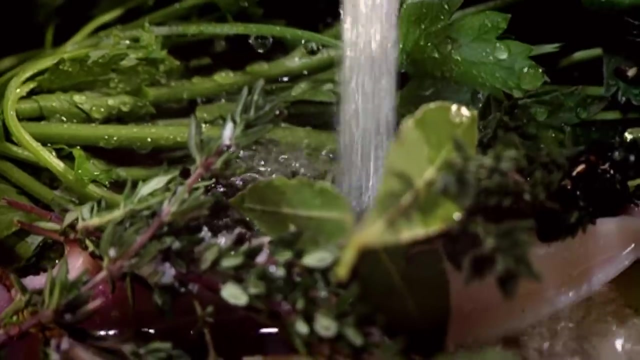 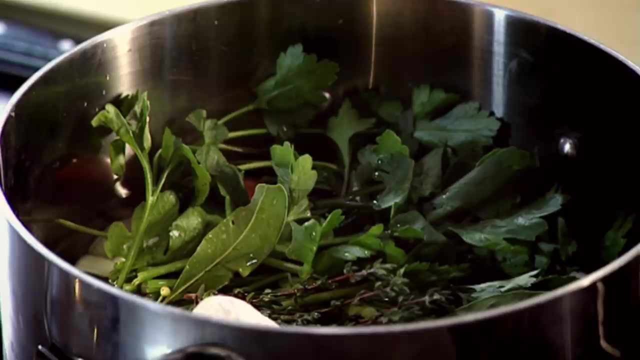 And a little pinch of salt And now just cover the vegetables and the carcass with cold water. Just cover the chicken and the vegetables, Bring it up to the boil as quick as you can. Now, as it comes up to the boil, 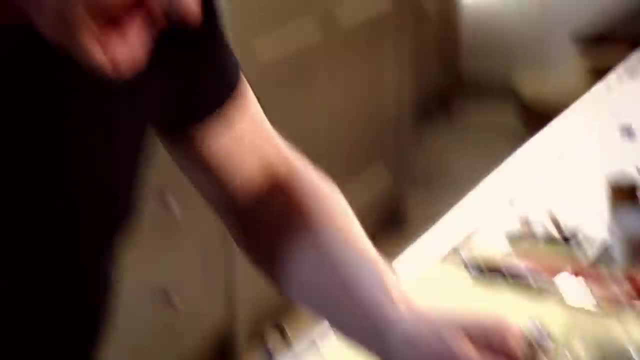 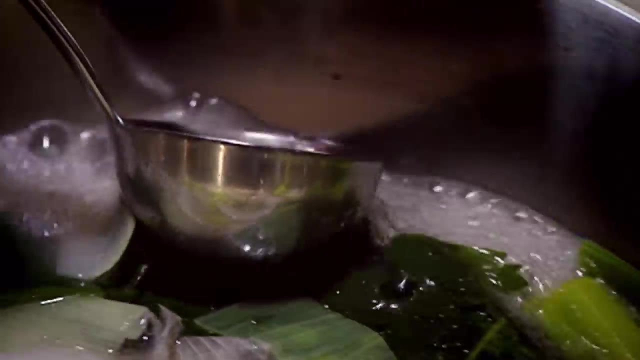 a really nice skim. Take the base of the ladle and swirl that around. That pushes All the grease and the impurities to the side of the pan. Then get your ladle and just tilt it If you don't skim all that off. 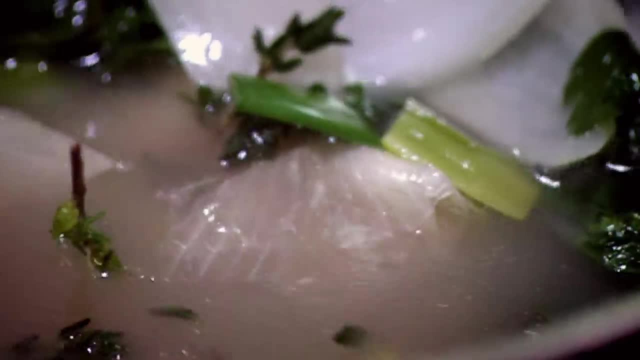 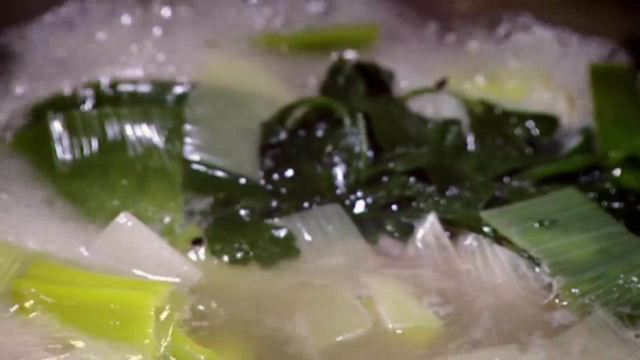 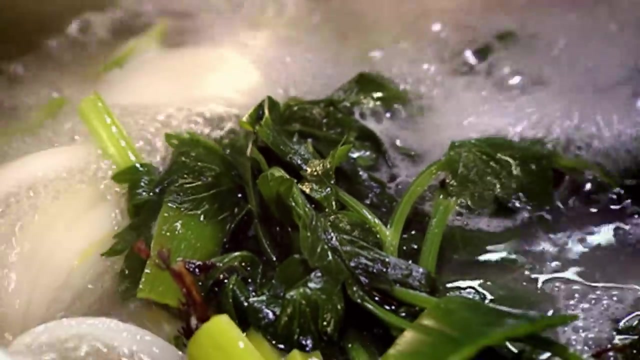 the stock becomes very cloudy. People's impression of cooking stock that it needs to cook for three, four hours at a time. This is one chicken carcass. Let that boil away gently for 30 to 40 minutes maximum. Now we're going to pass it off. 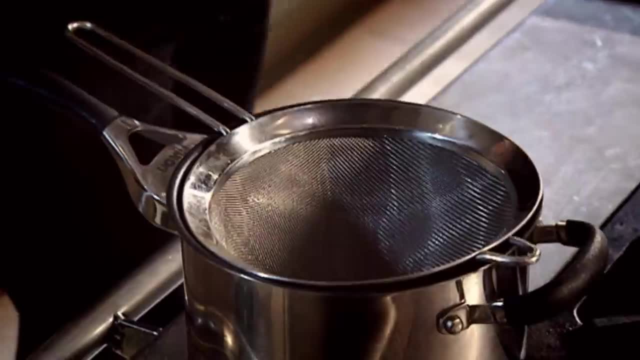 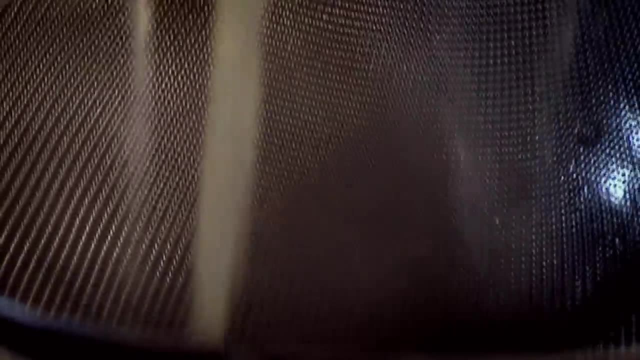 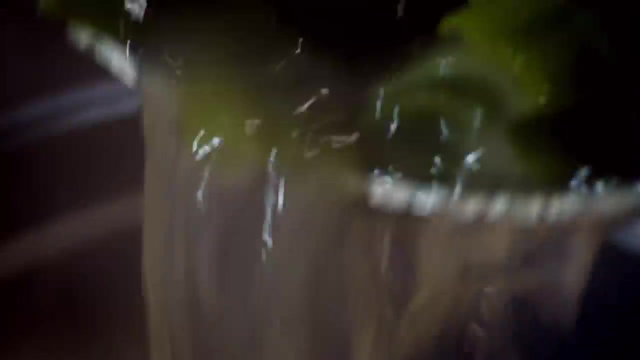 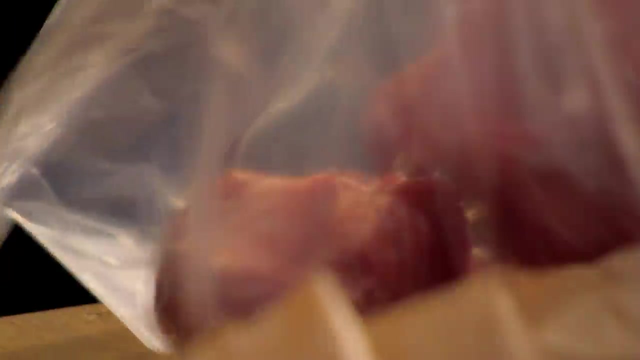 Take a sieve, Place that over the pan And then just pour that in. It smells amazing, It's aromatic, The color is absolutely beautiful And there you have the most amazing stock When you need to season meat in flour. 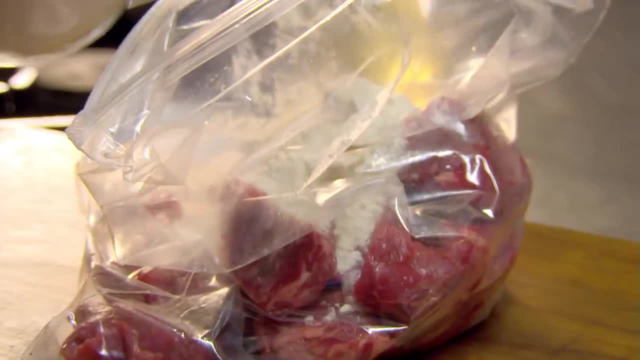 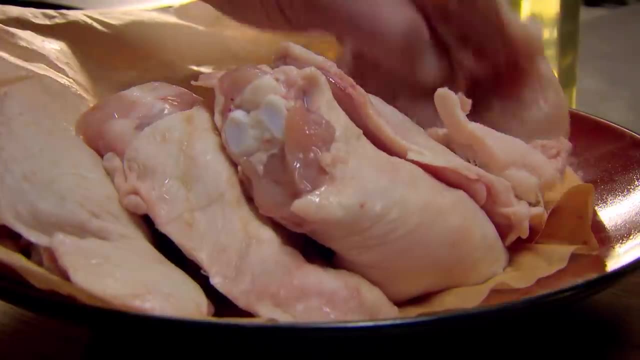 a great tip is to place it in a plastic bag to dust it evenly. Using flour also helps the sauce to get nice and thick during cooking. When browning meat, fry it in small batches. Don't crowd the pan, Otherwise it won't sear or color properly. 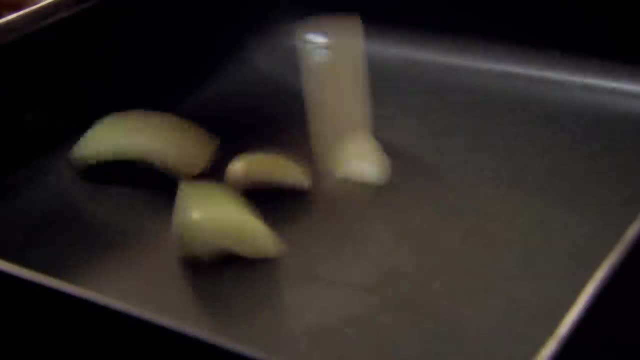 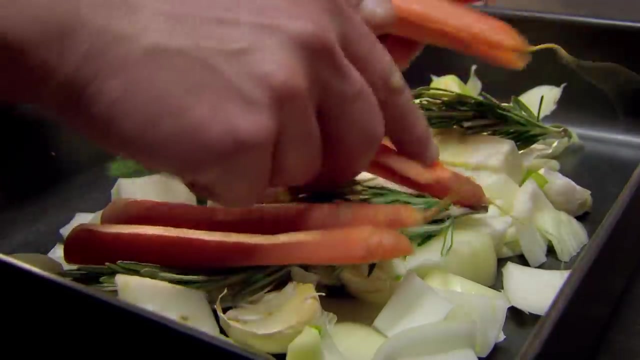 When slow roasting meat line the bottom of the roasting tray with chunky vegetables like onions, fennel and carrots, They act as a trivet to keep the meat from boiling in its own juices. Plus, the veg can be the base for your gravy later on. 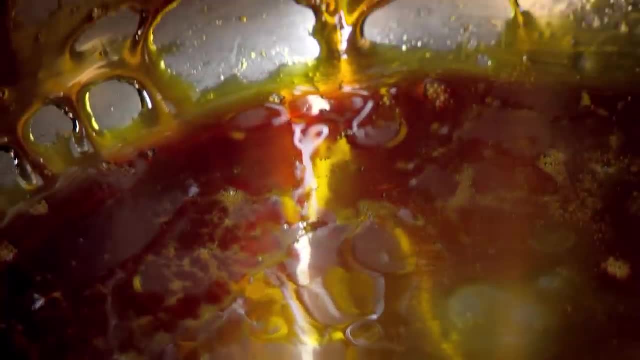 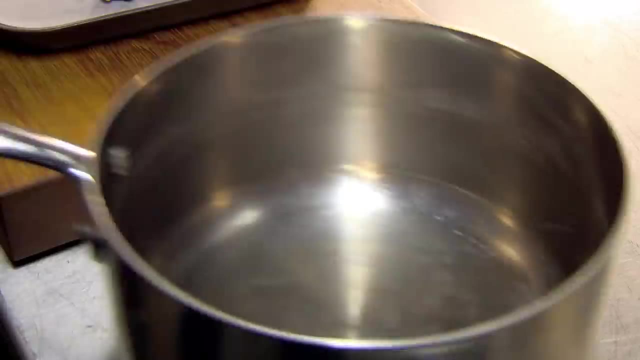 After slow cooking, baked on residue can be tough to remove, But if you boil water in the pan it will dissolve and break down. Then simply pour out and wash with soap and water. I absolutely love these peppers. Now. they have the most amazing, sweet, delicious flavor. 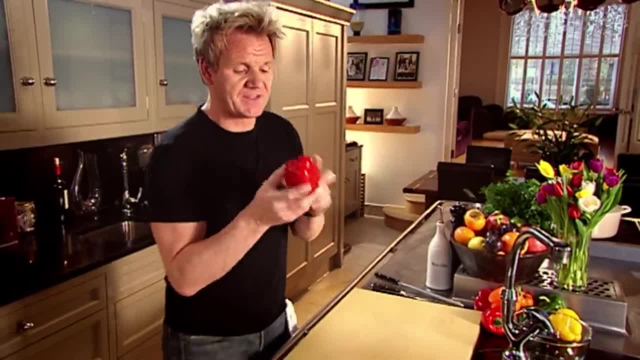 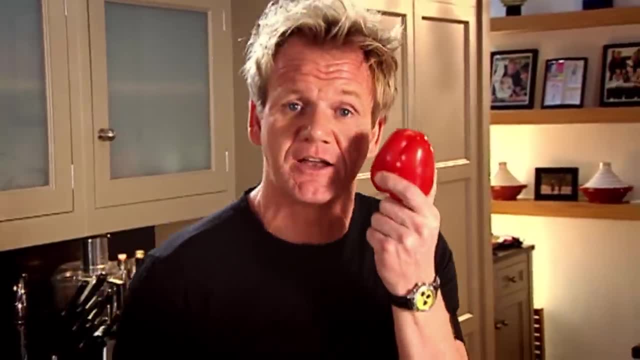 with a really nice crunchy texture. And the most exciting thing about the peppers is that they're just as delicious raw or cooked. To identify the perfect pepper, it must be smooth and firm and not a wrinkle in sight. Now how to cut the perfect pepper. 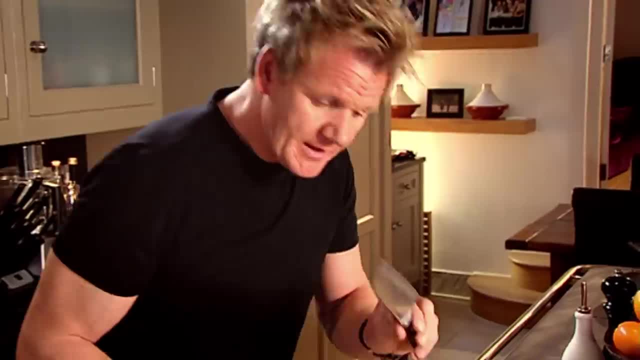 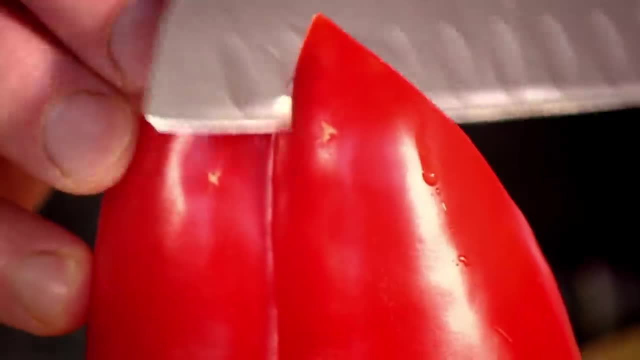 Stalk off pepper down and get the knife, Start from the top and slice all the way around. Basically, we're going to be slicing around the seeds. Look no faffing around like this little perfect Christmas tree of seeds. 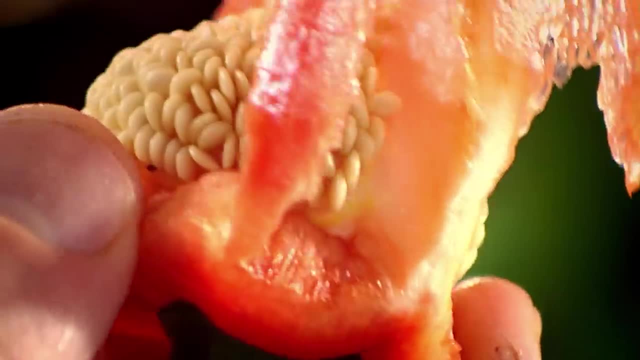 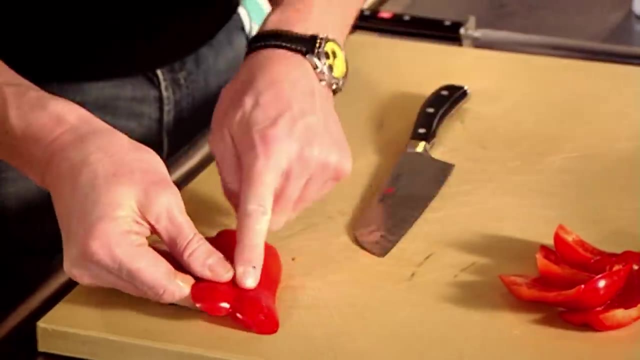 And you haven't got the mess all over your board. And, more importantly, it's twice as quick Discard that Now we're going to cut it into a julienne. Flatten the pepper Skin side down onto the board because it's a lot easier to slice through the pepper. 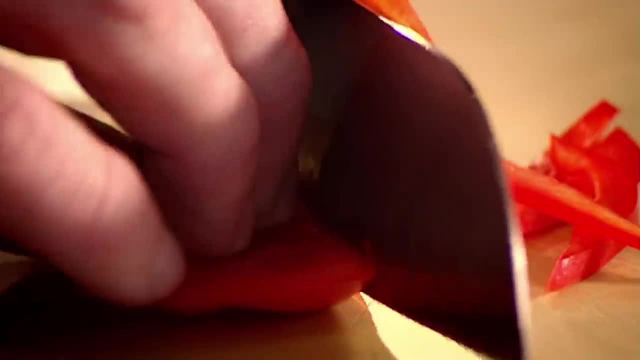 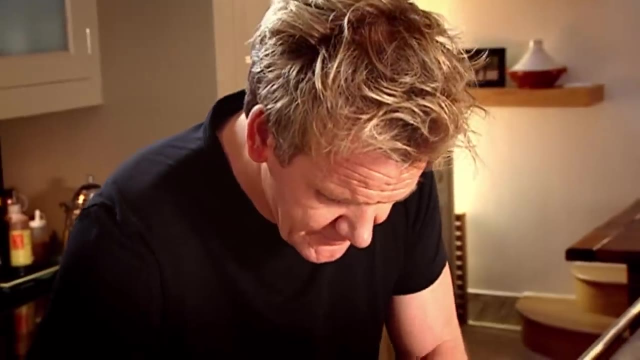 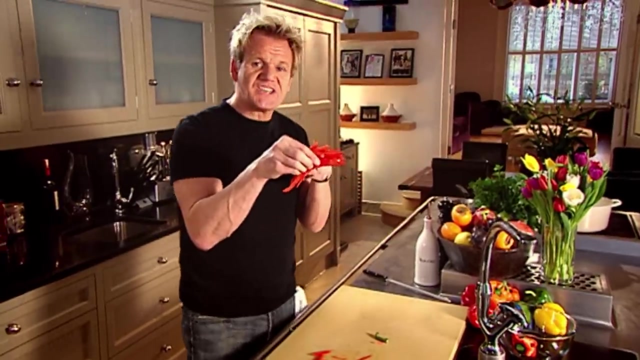 And just lift the knife up and down And basically, julienne is a chef's word for strips. These are absolutely perfect for sauteing And that's what we're looking for there: Crunchy, delicious and, more importantly, no seeds. 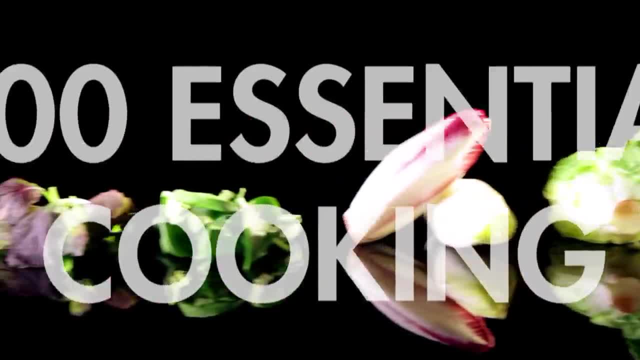 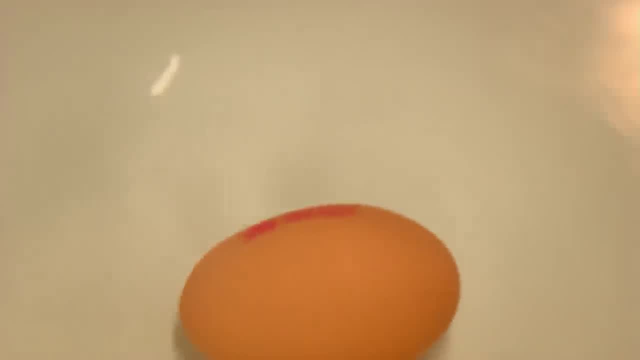 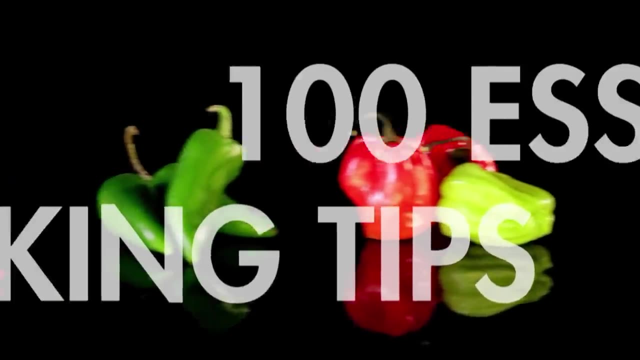 Beautiful. Many great brunch recipes start with a delicious fresh egg. My tried and tested way to tell if your egg is fresh is to simply place it into a bowl of cold water. A fresh egg will sink and a stale one will float If a small piece of shell goes into the bowl. 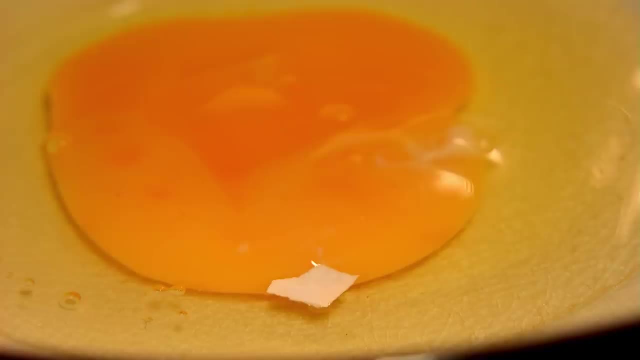 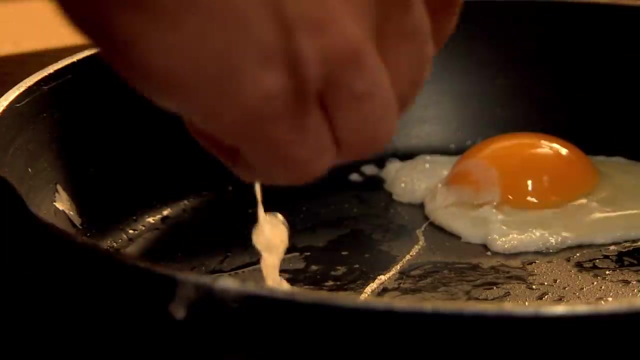 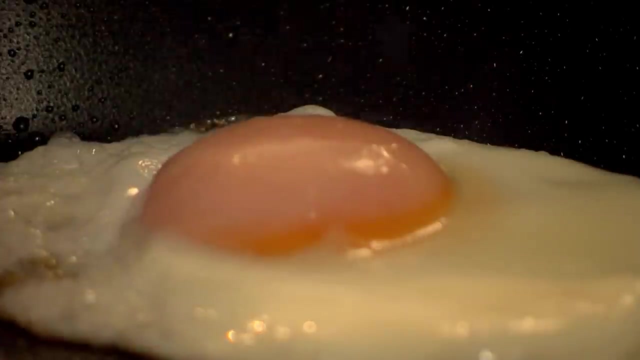 when you're cracking eggs, my tip for removing it is to simply use a larger piece to fish it out. It works like magic For prize-winning fried eggs. fry them in oil, adding a tablespoon of water, then cover. The water steams the top of the egg to perfection. 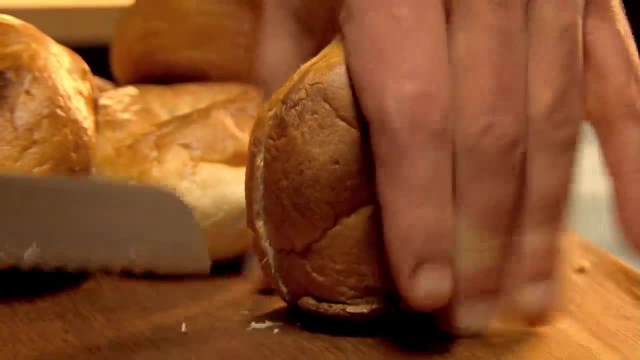 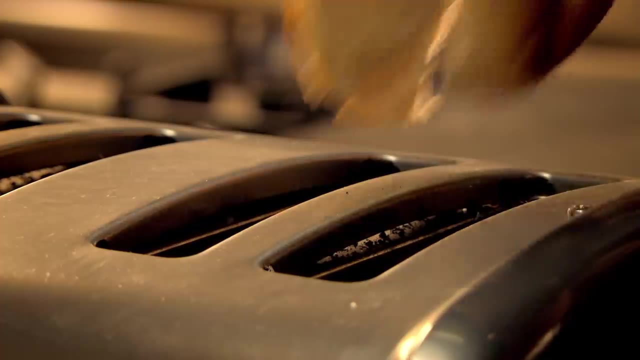 Toasted bagels are brilliant for brunch. My tip to make sure you always have them on hand is to stock up your freezer, But make sure you slice them first. That way you can pop them straight into your toaster. First up, how to peel and cut a mango: the easy way. 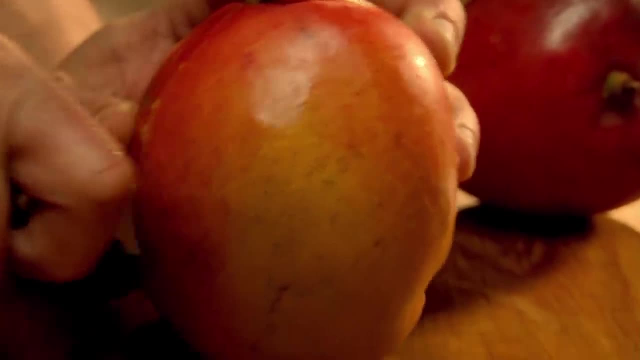 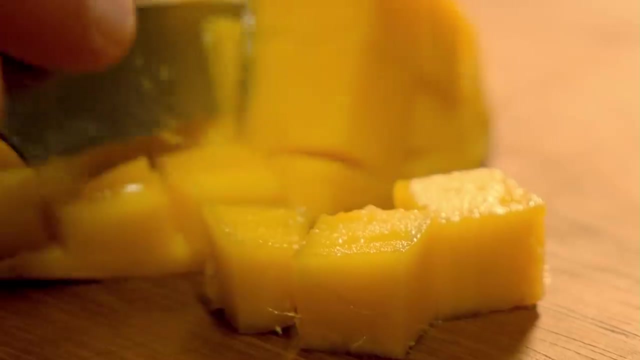 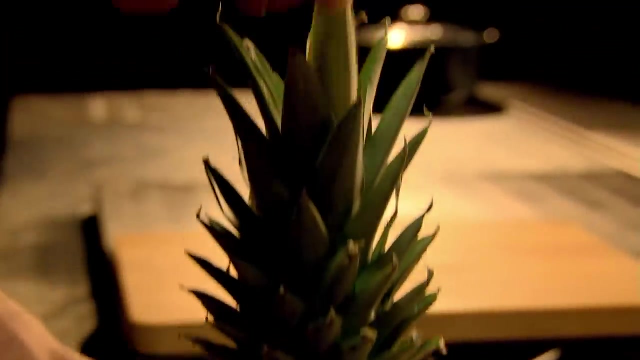 Holding its stalk end up. cut either side of the stone. Cut all the way into the flesh, making squares without cutting through the skin. Then turn it inside out and carefully cut your pieces off. A great tip to check if a pineapple is ripe. 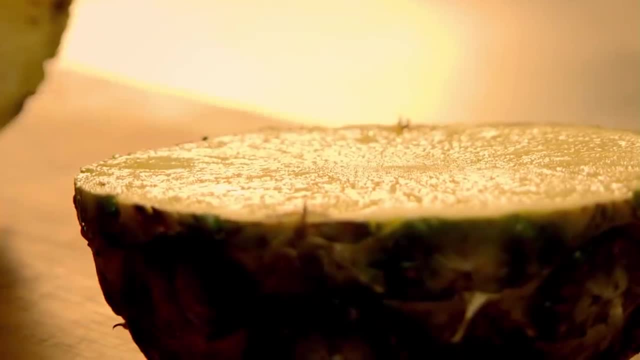 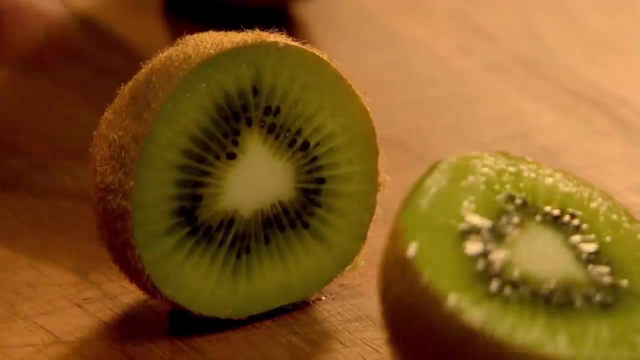 is to pull a leaf out from the top. If it comes away easily, it's ripe and ready for slicing. My tip to get the flesh out of a kiwi is to simply cut the fruit in half and scoop it out with a teaspoon. 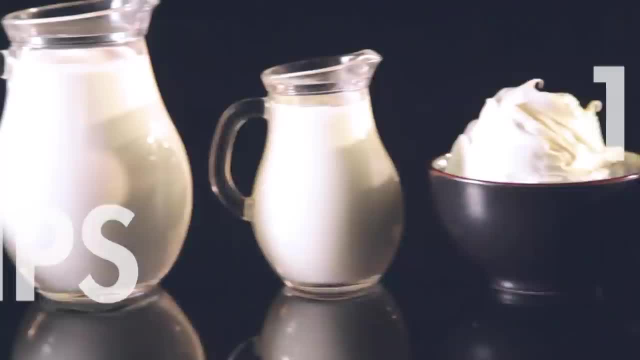 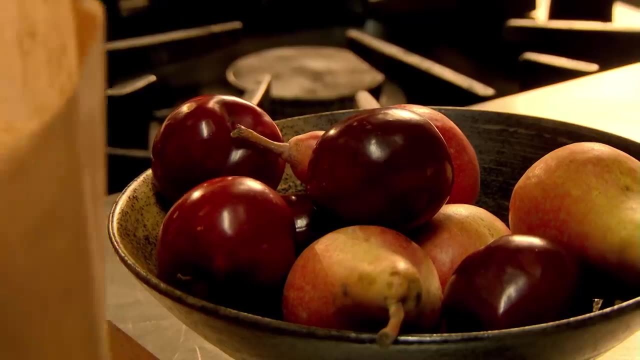 Try it. It really works. If you have fruit that's not perfectly ripe, the tip is to put a banana in a paper bag, then add your unripe fruit, Put it in a dark place and the banana will speed up the ripening process of the other fruit. 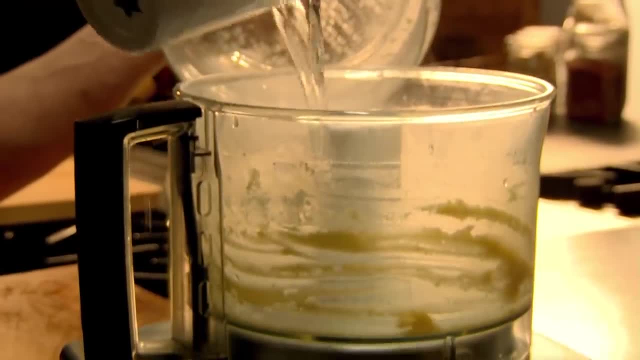 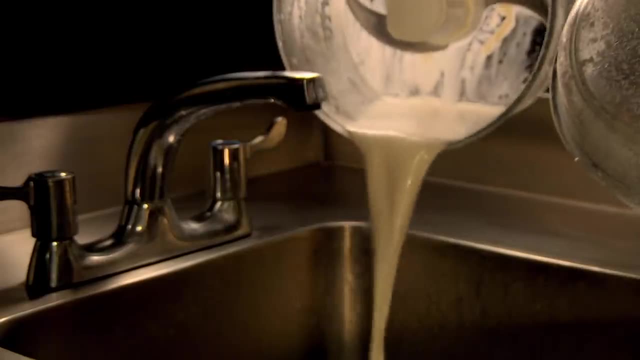 You can make a grapefruit puree to accompany a brunch pancake or a crumpet in a blender. To clean it afterwards, add a cup of warm water and run the machine for a few seconds. Empty out, then simply repeat with a drop of washing-up liquid, then rinse. 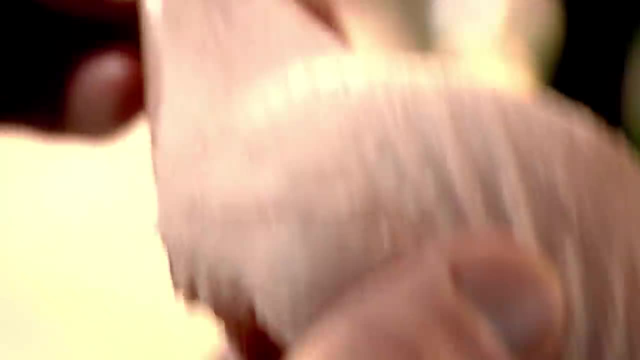 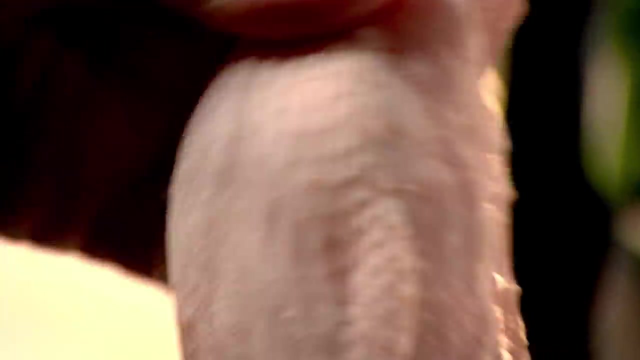 This has to be the most popular part of the chicken Now. it's very versatile, incredibly tender, very lean, hardly any fat whatsoever. The secret is cooking it without it becoming dry. The first thing is to season it properly, Both sides. 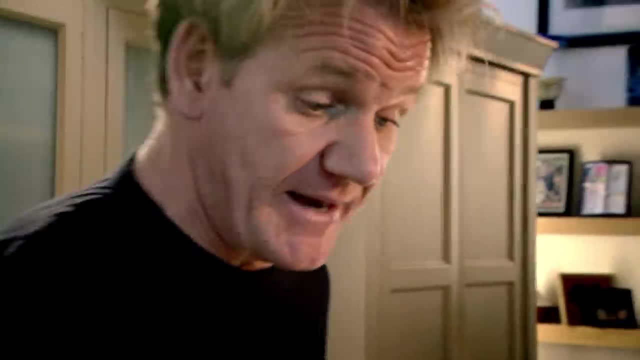 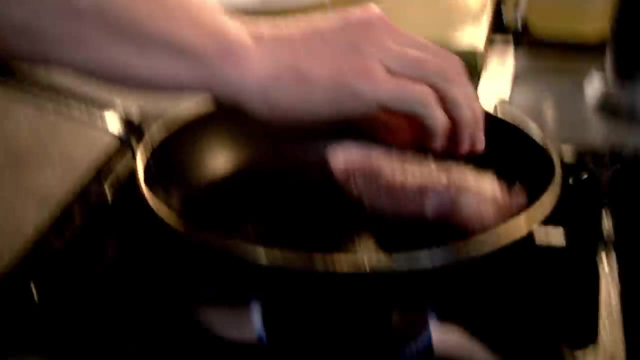 Two tablespoons of olive oil. Get the pan nice and hot. The secret now is to get a really nice colour on the skin. Really nice colour. No colour, no flavour. Skin side down. Tilt the pan so it cooks the back of the chicken breast. 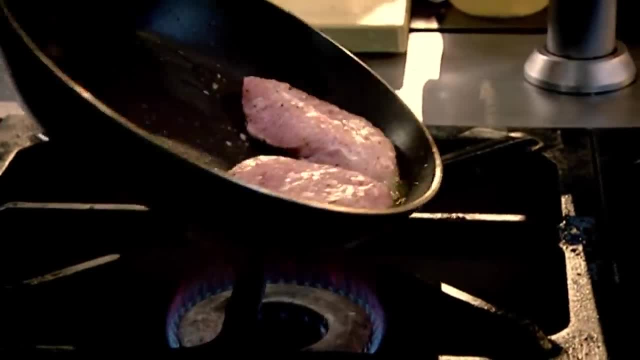 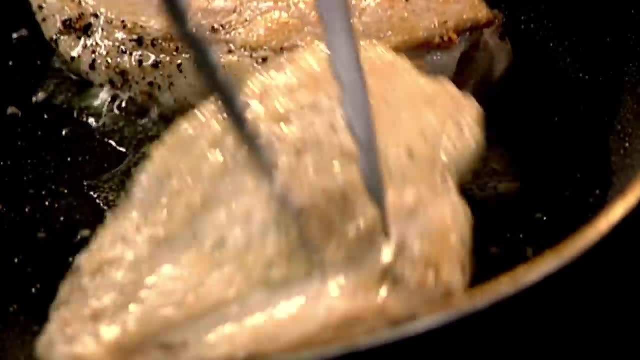 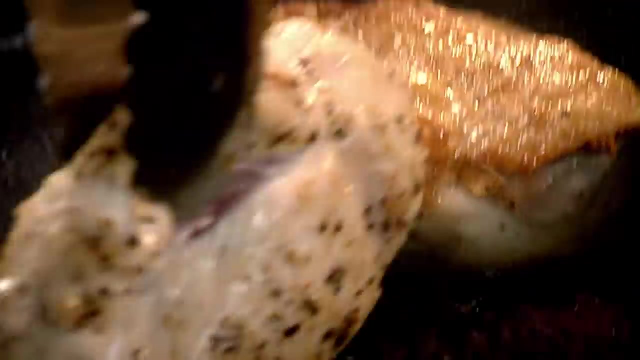 where it's really nice and round and very fat, Let the pan do the work. Chicken breast normally takes between sort of 10 and 12 minutes to cook properly. Now we've got the colour on the skin. The skin's nice and crispy. 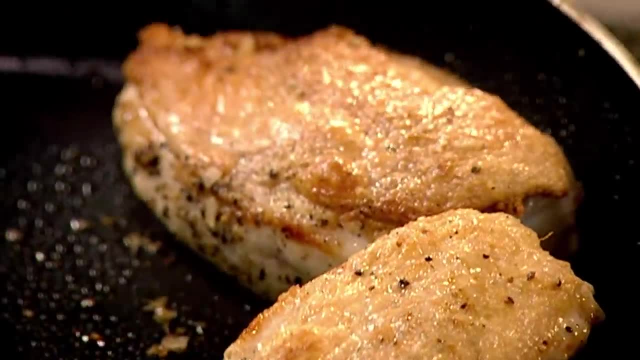 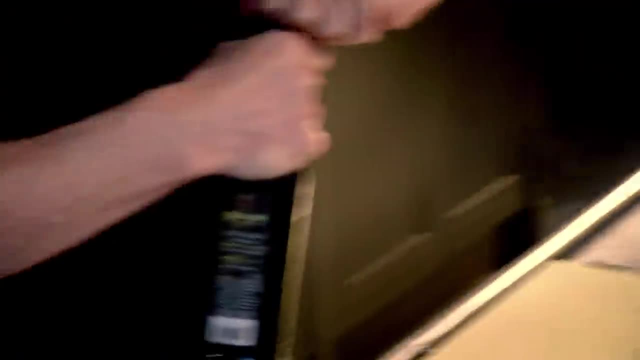 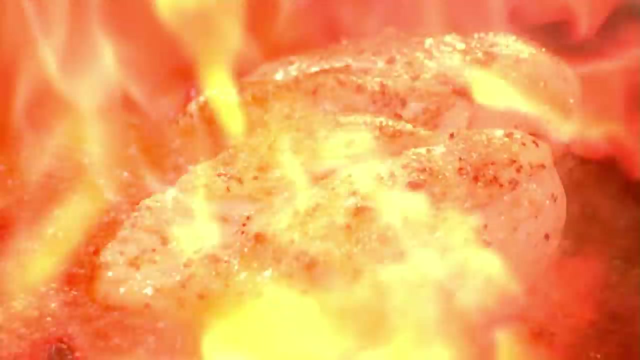 We're going to deglaze the pan. Deglaze with masala. Now, masala's a sweet, fortified Italian wine. You can also use white wine Masala in Flambe. Burn off the alcohol, which gets rid of that really sort of harsh alcoholic flavour. 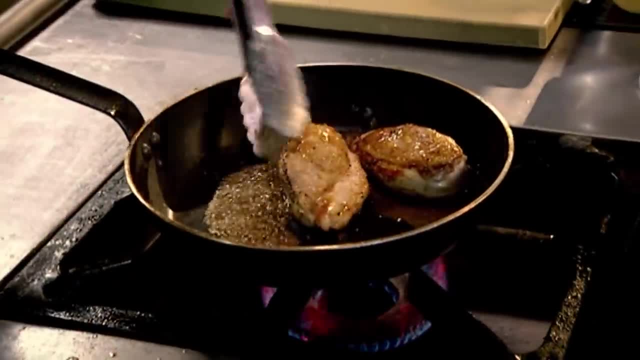 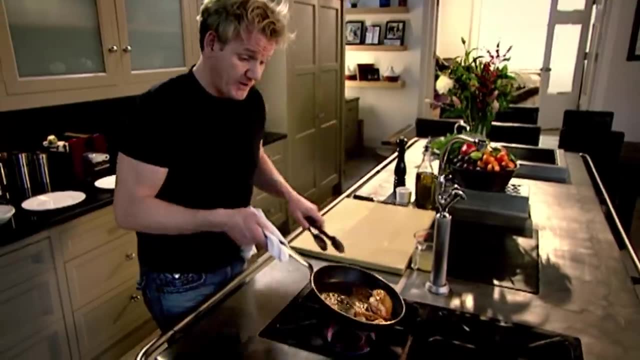 Roll the chicken around the masala. Deglazing the pan basically means washing it, Deglazing the pan And lifting off all that flavour stuck to the bottom of the frying pan and putting it into the sauce. Now, chicken stock: Bring that up to the boil. 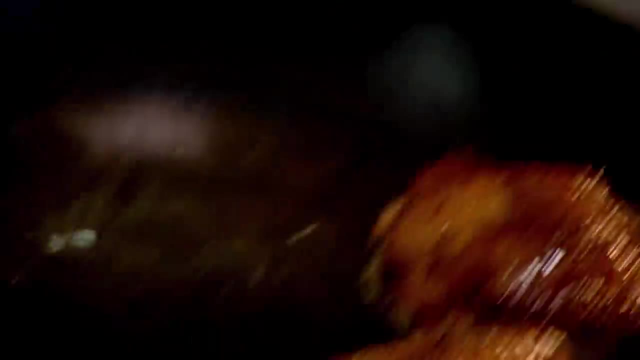 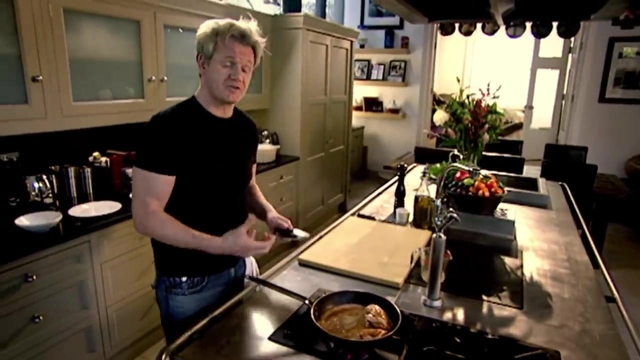 and let it simmer for three to four minutes. Really important to leave the chicken breast skin side up. The skin's nice and crispy and it's important now that the chicken cooks from underneath. As it starts cooking it absorbs the stock, So in the centre the chicken stays nice and moist. 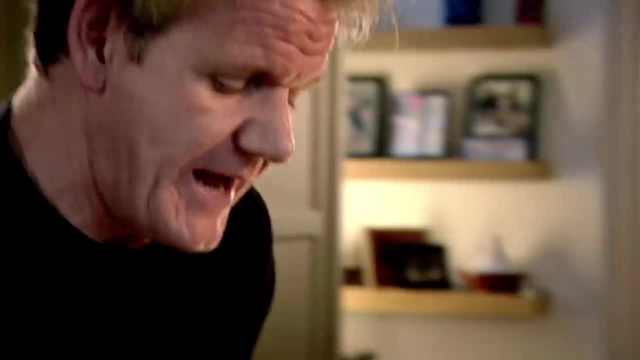 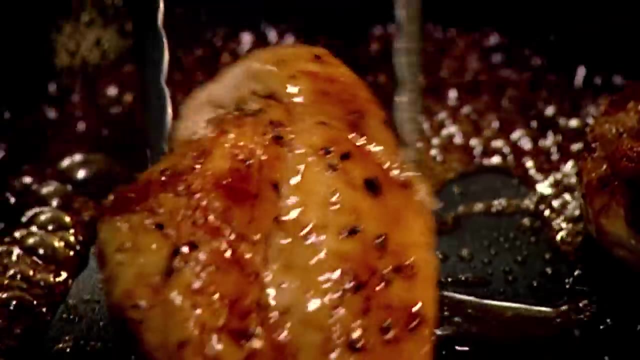 Now the stock and the masala's reduced down, Grab the confidence to allow it to almost disappear. And look, The combination between the masala and the chicken stock is quite sweet, so it finishes the chicken with this really nice, delicious glaze on top. 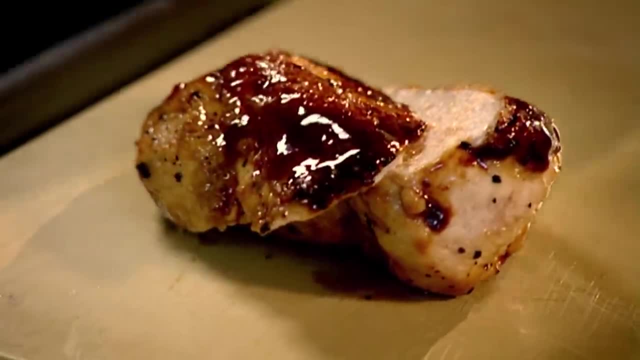 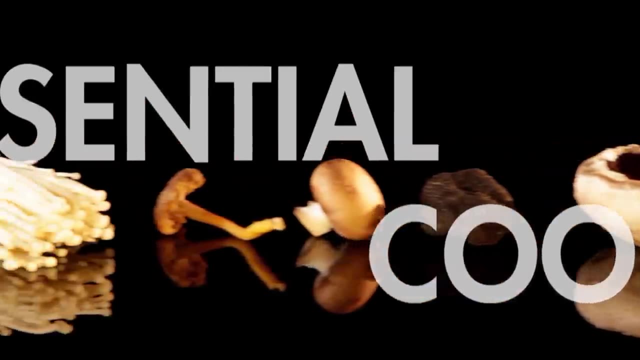 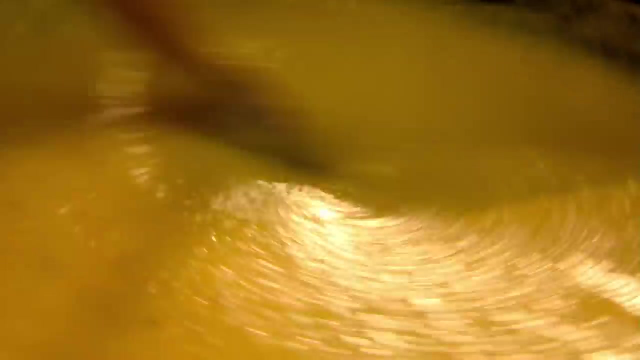 And there you go: A delicious, succulent chicken breast with the most amazing flavoursome skin. Phenomenal Soups make stunningly simple meals. My tip for adding incredible depth of flavour is to always keep your leftover parmesan. Store them in the freezer, then add to the pan. 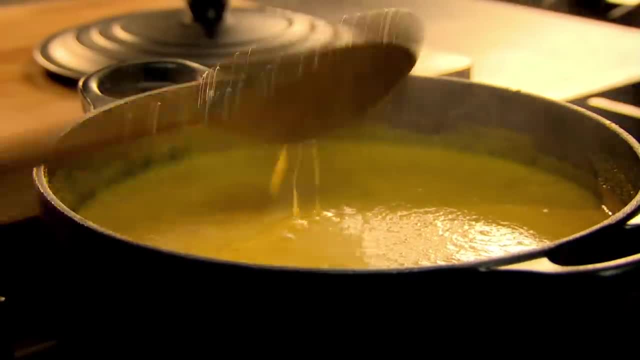 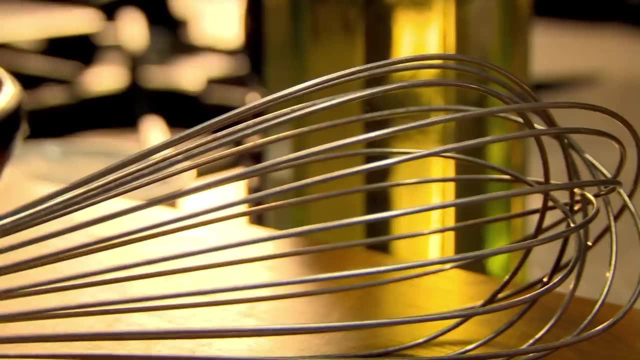 as the soup cooks and leaves to infuse, Then remove before serving. It's less waste and more taste. Another tip to take homemade soup to the next level: whisk in cubes of cold butter just before serving to get a glossy, velvety texture. 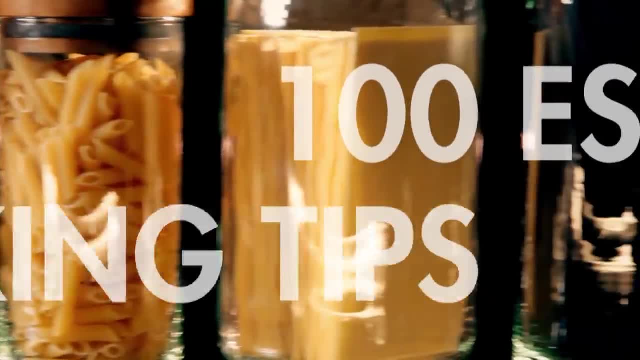 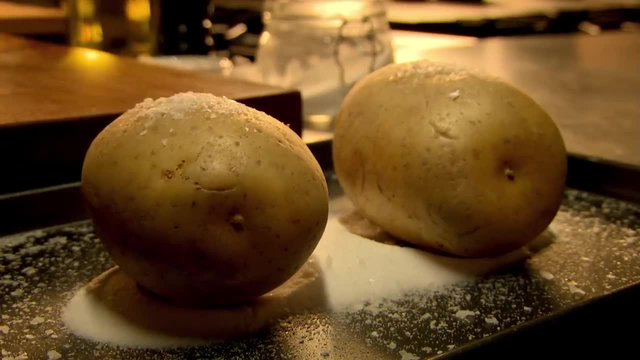 and a beautifully rich taste. Another fantastic standard for a fuss-free weekend eat is the classic baked potato. My tip for a great crispy skin is to use salt to your advantage. Simply add it to the outside before cooking and the salt will draw out the moisture in the oven. 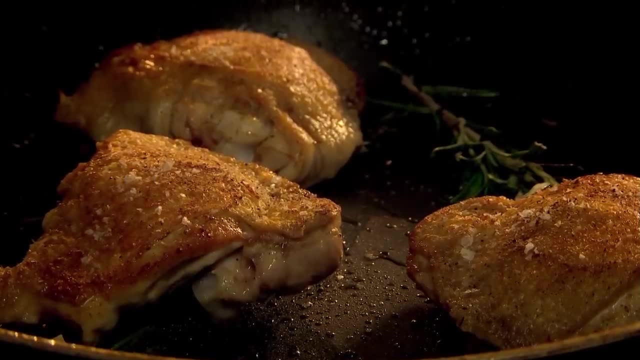 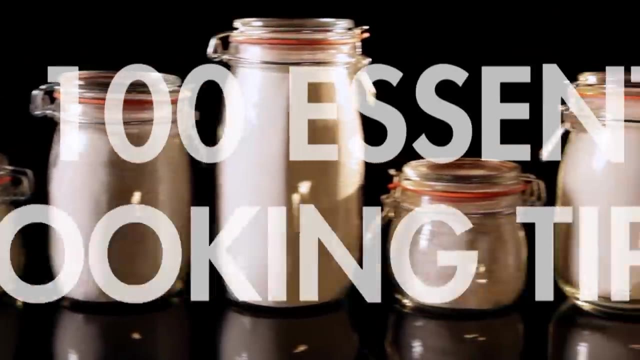 as it bakes. A touch of salt gives you an amazingly crisp skin on chicken and fish too, as well as highlighting the flavour. Home-roasted nuts make a delicious TV snack. My tip for peeling them with ease is to simply toast them in the oven for about ten minutes. 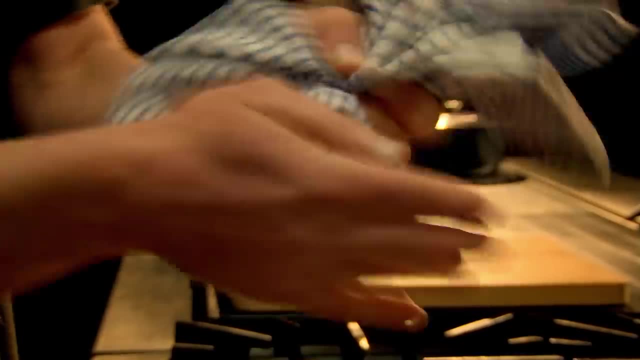 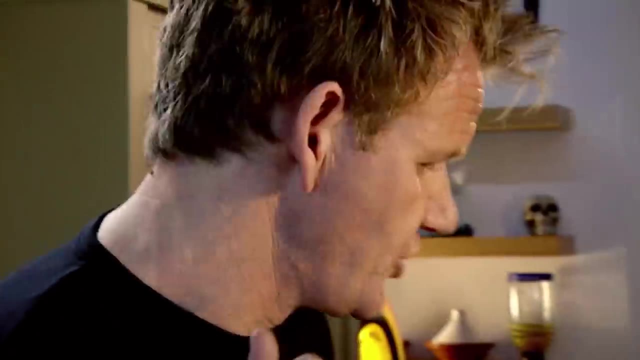 wrap in a tea towel and rub until the skins are removed. Perfect sprinkle with sea salt and so with a glass of wine. Chopping herbs: The secret is to chop them, not bruise them. Now, basil: This is a soft herb, so treat it with some respect. 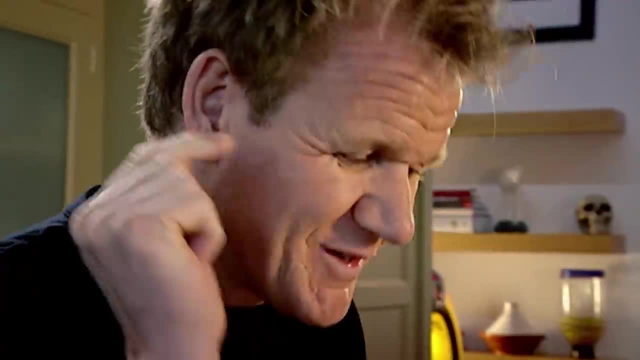 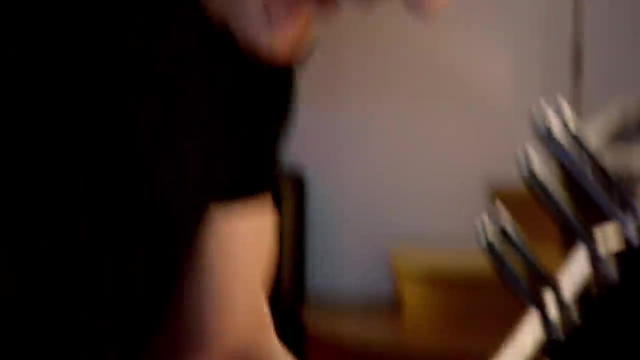 When people go mad chopping herbs, all the goodness comes out on the board. I want the goodness left inside the basil. Place them all inside one another, with the largest leaf at the bottom, And it's almost like rolling a cigar: Large one at the bottom, small ones in the centre. 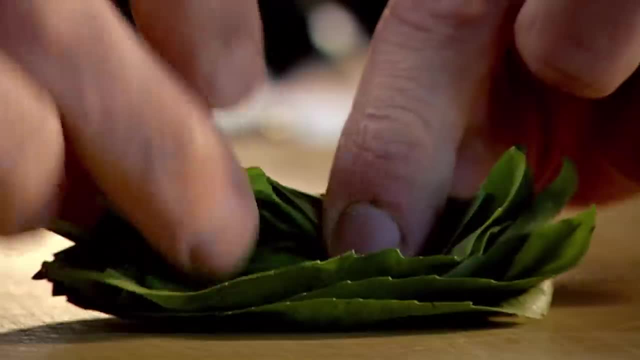 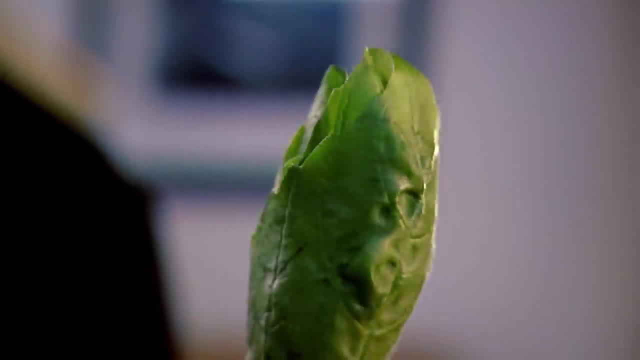 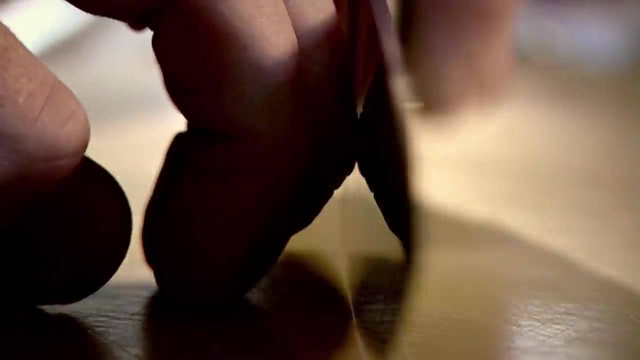 And then look, place them down together and just roll them nice and gently, Don't bruise them. Step one Rolled, ready to slice Sharp knife. imperative Fingers tucked in The bottom part of your knuckle is the guide between you and the herbs. 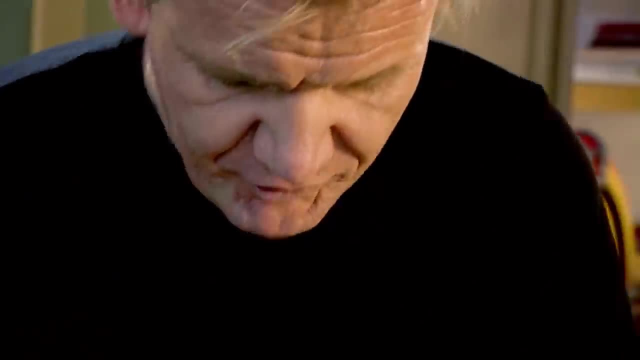 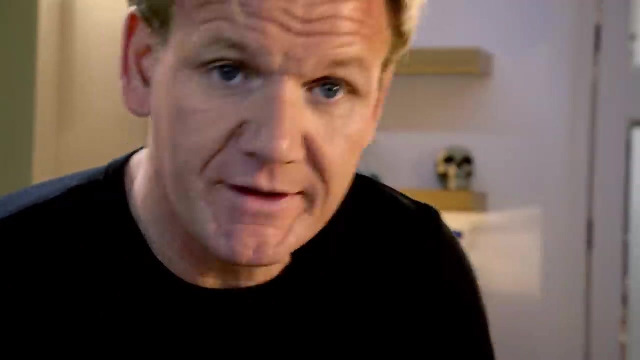 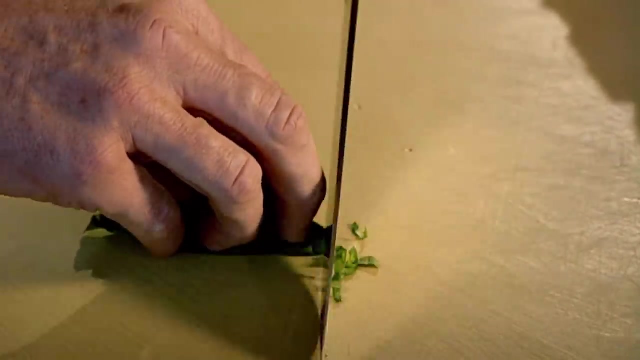 That there stops you from cutting your finger. Really important to get comfortable with the knife and just practise rolling the knife across the board and relaxing that wrist. It's all in the wrist action. So herbs up, Fingernails tucked Underneath. 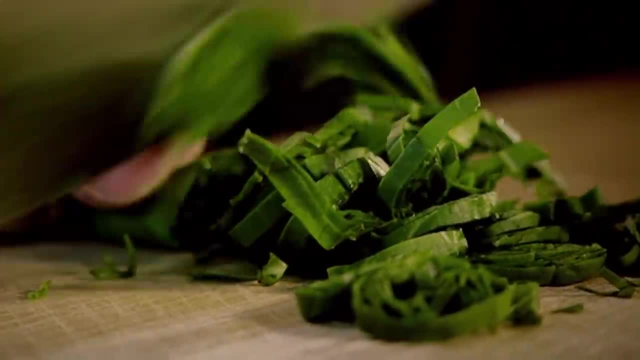 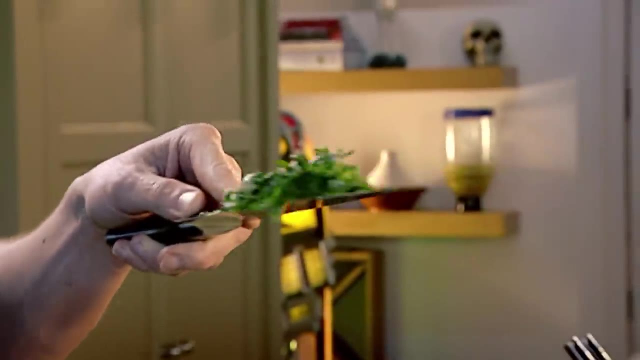 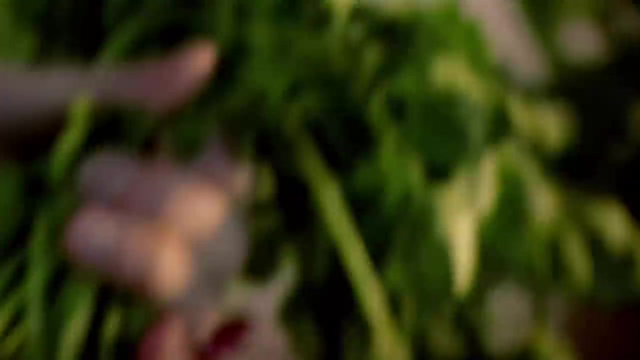 And just up and down, Up and down, And there you have a chopped basil that's not bruised and smelling very fragrant, Right, coriander. So you get the bunch of coriander, Hold it down And just lightly shave the leaves off the stalks. 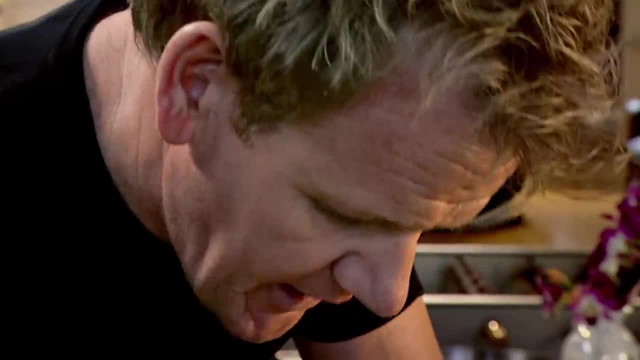 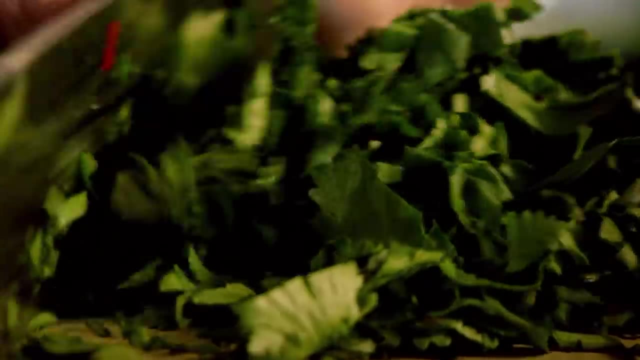 Bunch them up together And just again, let the knife do the work. Tuck the fingernails in and just chop, once And once. only, Don't hack it, Just chop it. You can always identify when you've bruised a herb. 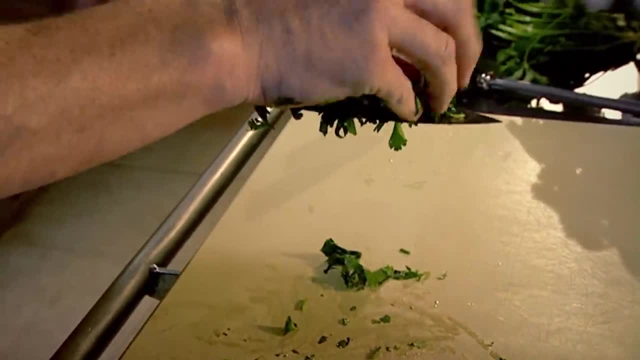 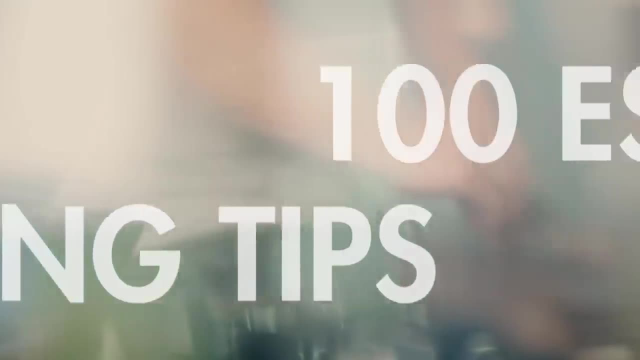 When you've removed the herbs off the board and there's a big green patch, Mmm Full of flavour, And none of the goodness is left on the chopping board. A great tip for using leftover herbs: simply chop finely, mix into butter. 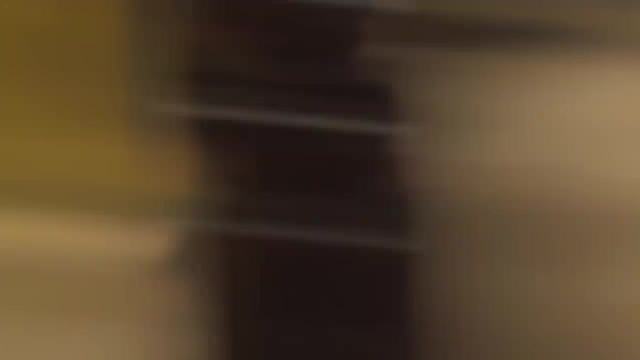 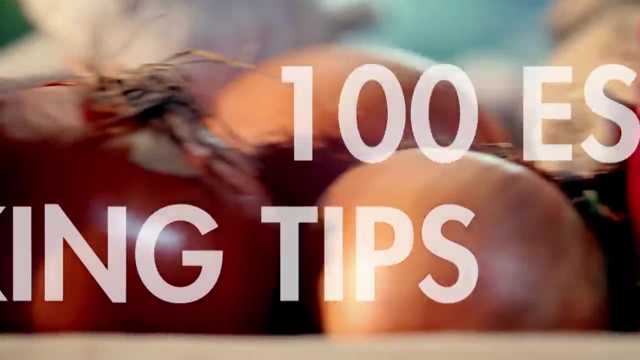 roll up in cling film and freeze. Then when you want a herby hit, cut into slices and melt over steaks, chicken or veg. Asparagus is great for a simple supper To prepare. always remove the lower woody stem by gently bending. 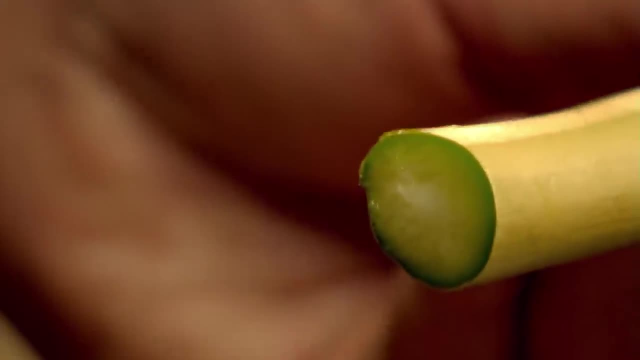 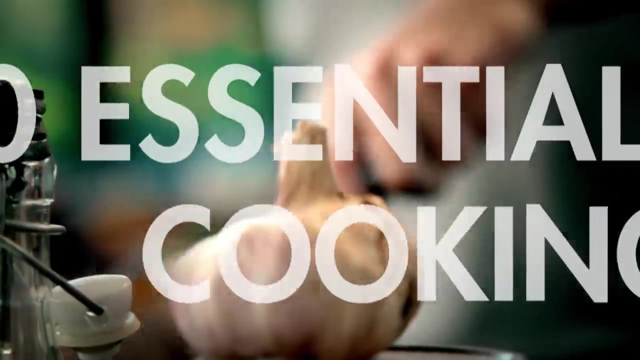 And the asparagus will snap at the perfect point. Then boil or steam and serve with a little of my herb butter. For a cracking soft-boiled egg: simply place your egg in boiling water, add a splash of vinegar and cook for exactly three minutes. 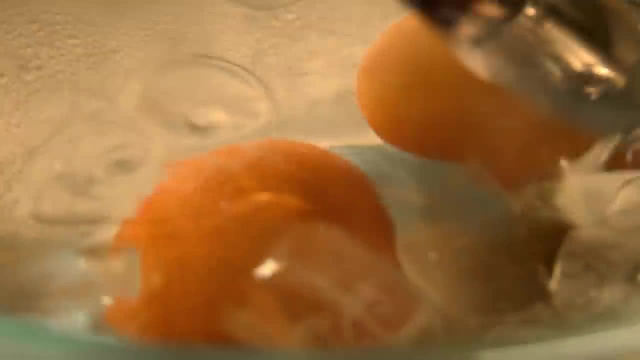 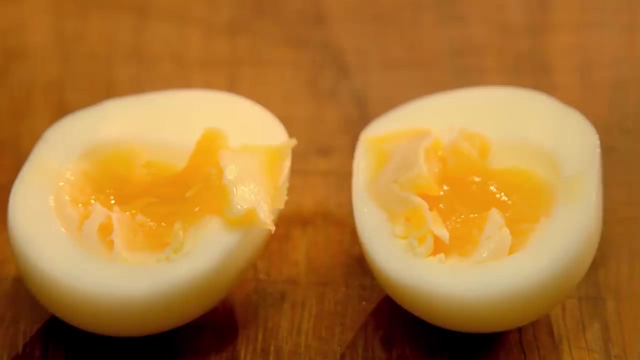 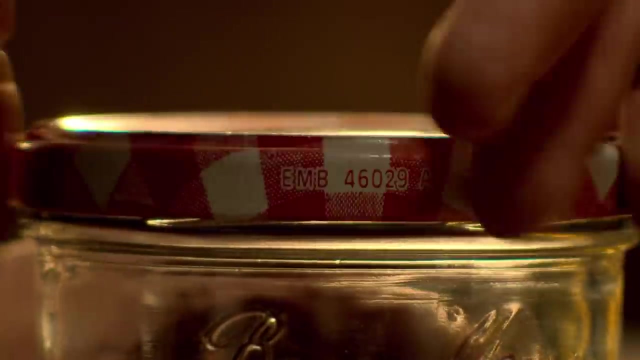 Then plunge into ice water. The vinegar helps the shell peel off easily and the ice water stops the egg from cooking, giving you the perfect runny yolk For fuss-free salad dressings. simply add the ingredients into a jam jar, Screw the lid on tightly and shake to combine in seconds. 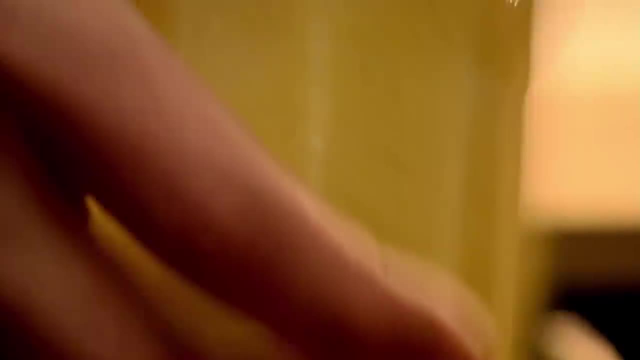 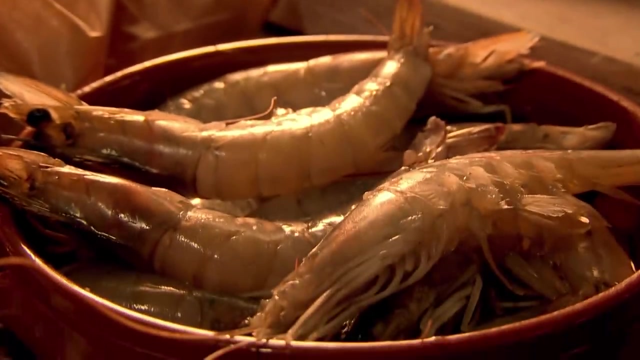 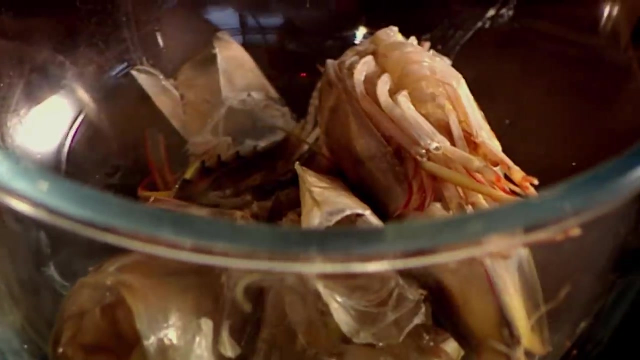 There's no need to wash up a whisk and the jar's ready-made to store any leftovers With how to prepare prawns. To prep it, get the head and twist, Keep hold of those heads, make the most amazing stock And then, with your thumb, get underneath the shell. 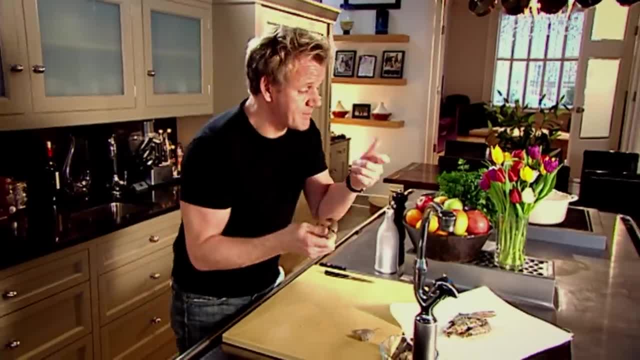 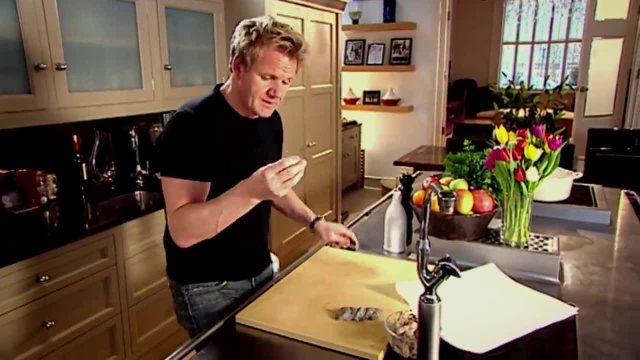 and just peel off that beautiful little layer. Now, with your thumb and your finger, push and shake and look- The whole tail comes off. You don't have to peel the whole thing From there. get your knife and just gently cut the surface of the prawn. 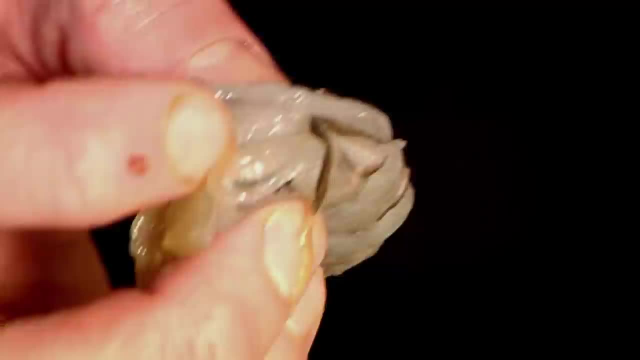 And what we're looking for there is that little dirt sack That's got to come out, Otherwise if you cook the prawn with that sack in there, it's crunchy, it's not very nice and it ruins that sweet flavour. 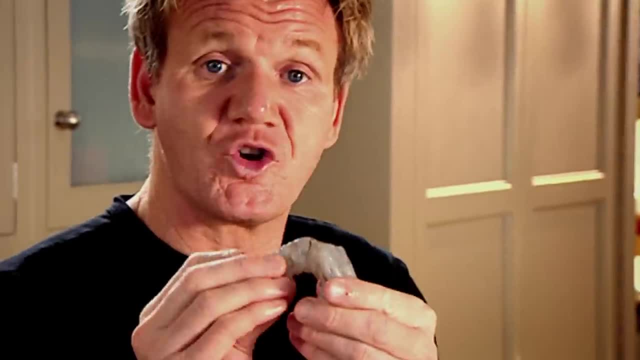 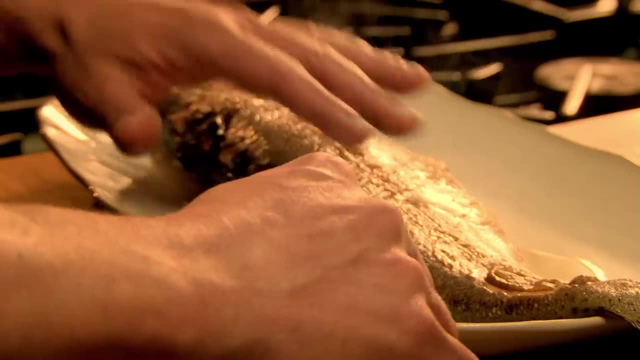 And there you go, The most amazing prawn ready for cooking. Serving whole fish always makes an impact. Here's how to fillet it at the table: Run a knife along the backbone, Remove the skin And carefully lift off the portions of flesh. 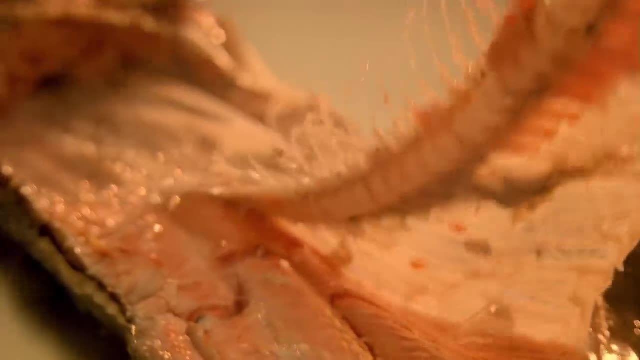 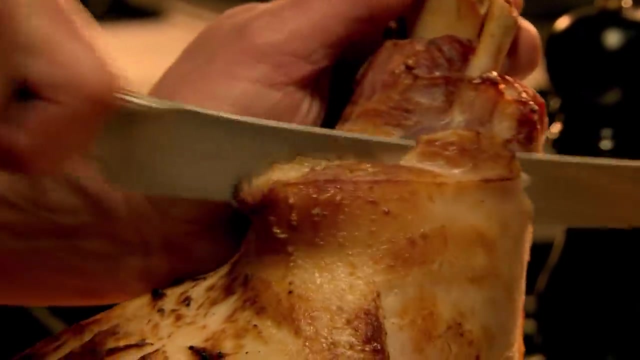 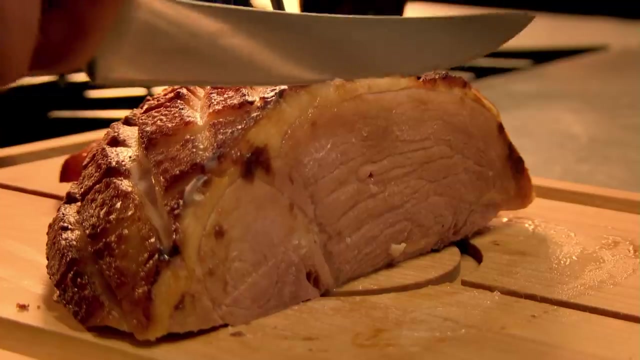 using a fish slice. Then just lift off the backbone in one careful movement. Whole hams are always impressive. To carve one easily. hold the ham by the bone and cut down the meat as close to the bone as possible. You can then lay your cut ham flat on the board. 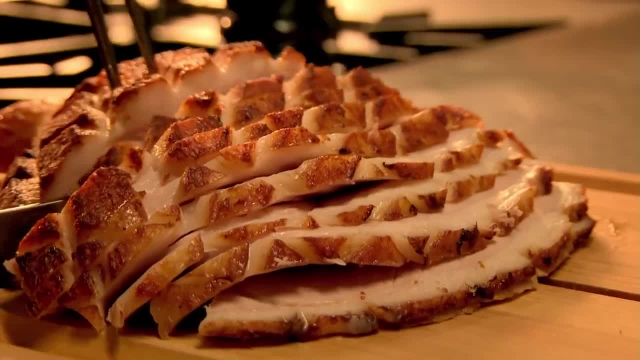 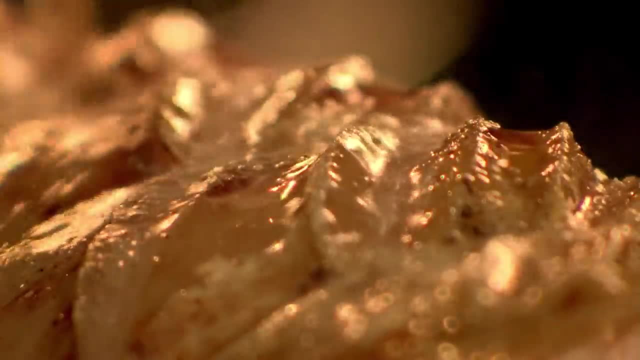 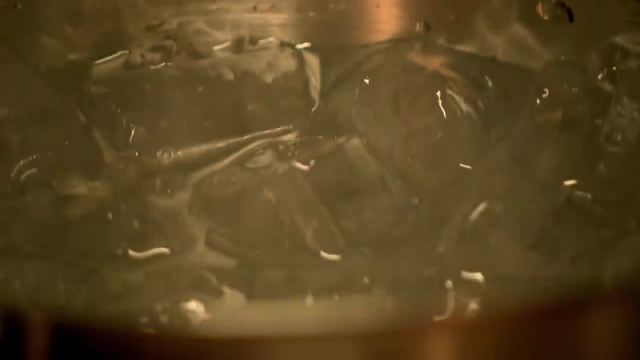 making it nice and easy to slice thinly and evenly. For perfect pork crackling, pour over hot oil before roasting in the oven. It'll come out beautifully crisp and crunchy. And when you need to chill wine fast, simply add a large handful of salt to your ice bucket. 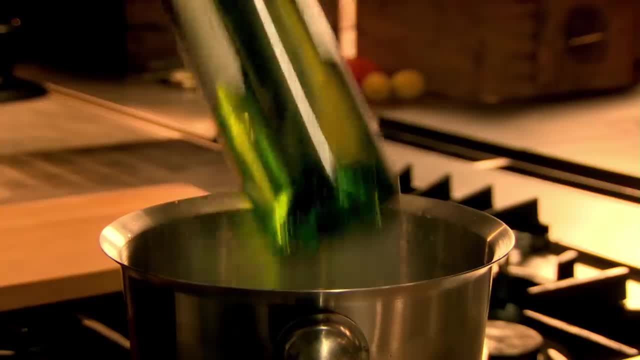 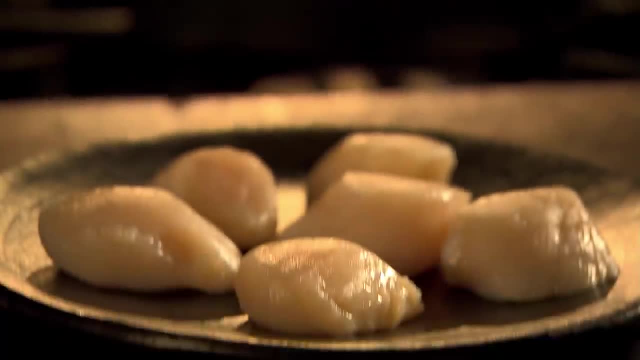 The salt reduces the freezing point of the water, which will chill your wine in six minutes. flat Scallops are a fantastic ingredient when you want a special salad that really impresses. Here's how to prepare them. Do not be intimidated trying to get the scallop out. 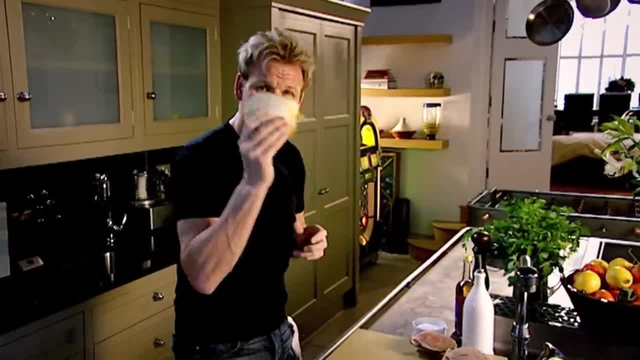 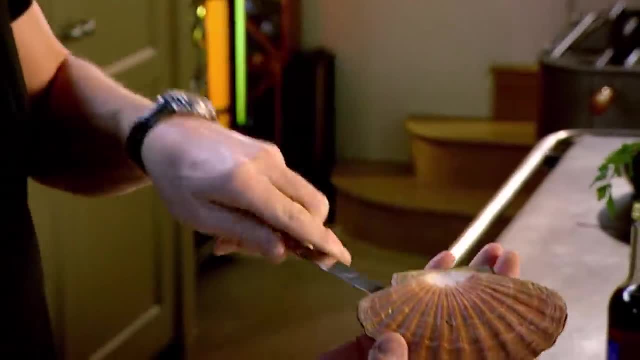 I'm going to show you how easy it is to take them out and how much more exciting it is to get them fresh in the shell. So just place the dessert spoon and a blunt knife, Put the knife in To the bottom And you just twist. 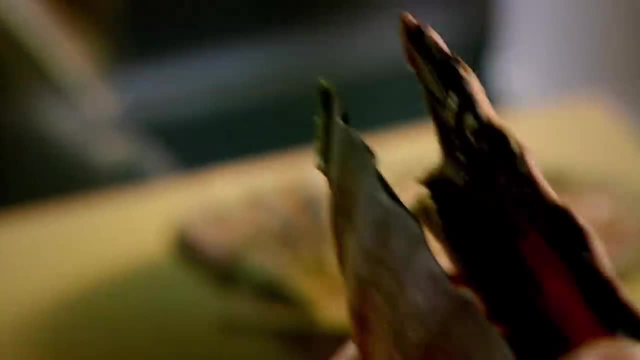 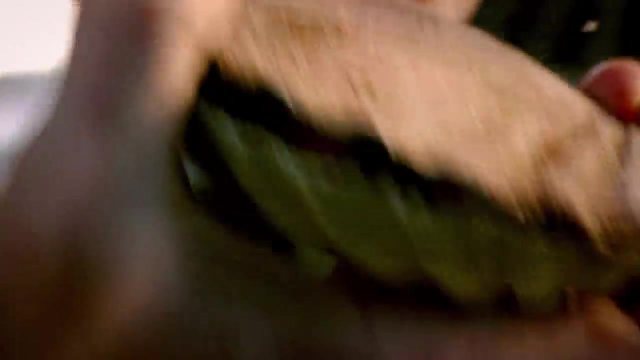 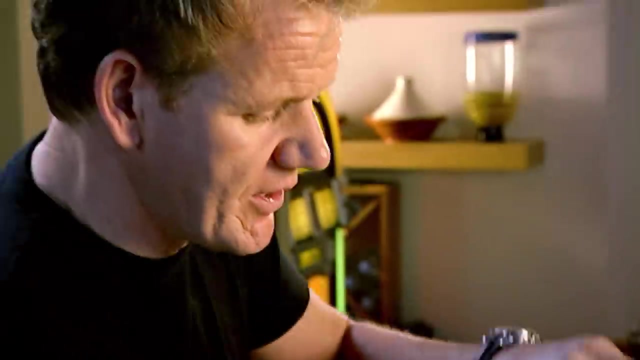 Open. Tilt the knife up so it doesn't cut into the scallop meat. Run the knife from the top to the base Off with the lid- No flesh on there, And then from there That's called the scallop skirt. 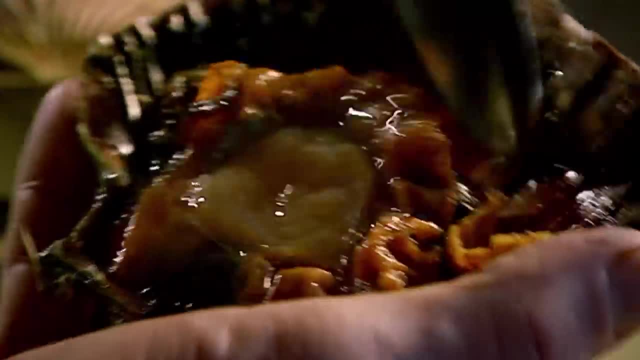 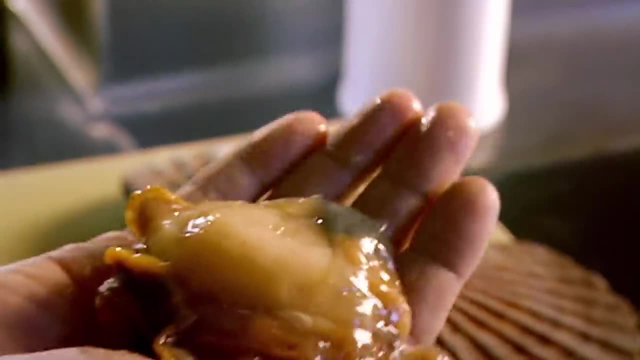 All you do is just peel that forward and get the spoon to run down the back of the shell And the idea is to remove that little bit of muscle that holds the scallop onto the bottom shelf. Bang It pops out. That's the top.